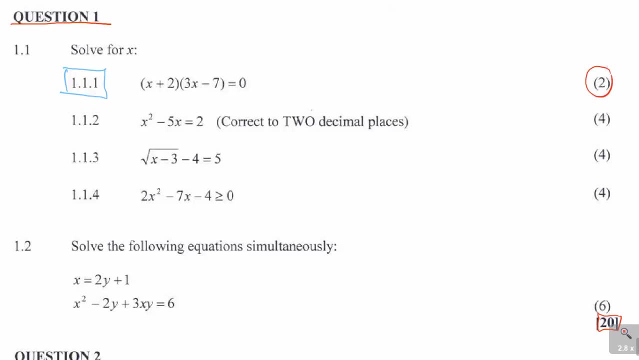 question is two marks, as you can see. So that is what they bring usually at the beginning. So I'm just going to solve it. It says X plus two, And the other one other bracket is three, X minus seven, And then this is equal to zero. So you're supposed to solve for X. So the good thing is. 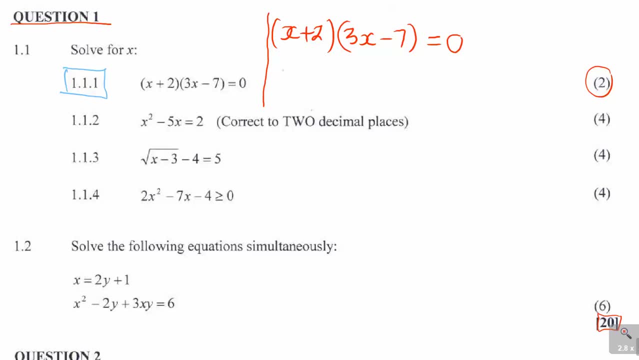 already. it is in brackets. So you are saying: either the first bracket, which is X plus two, is equal to zero, or the second bracket, which is three X minus seven, is equal to zero. So that's how you approach it. So in the first one you take two, transpose two to 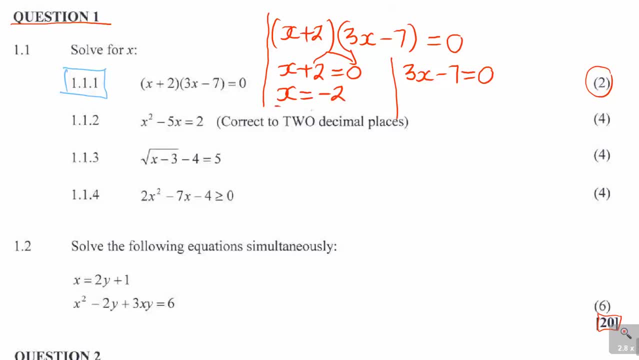 the other side it will be: X is equal to negative two. That's the first value. Or in the second one: also transpose: the negative seven will become positive seven. So you'll have three. X is equal to a positive seven. Now the three and X are multiplying there. you can see that. So the only 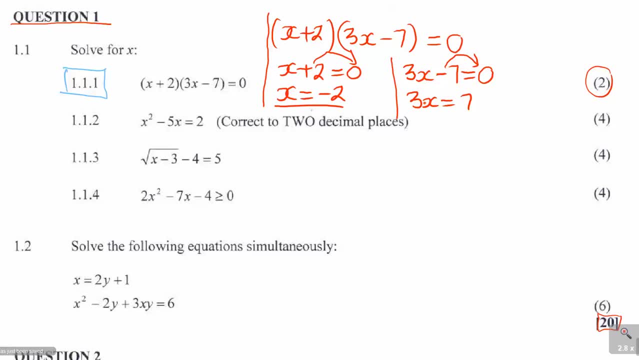 way to separate three from X, since it's multiplication three dot X. you can do the opposite of multiplication, which is division. So you divide by three, you divide by three. please take note that three cannot be, cannot cross the equal sign to become from positive to negative. That is wrong. you can only divide by three. 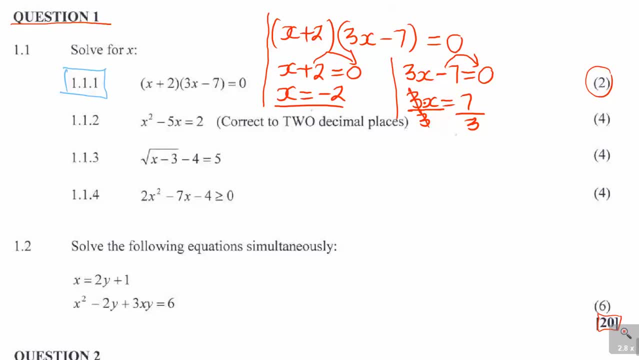 because three and X are multiplying. So you do the opposite of multiplication, which is division, and then you get the value of X as seven over three. So this is how you solve for X. in the first one is two marks. So what you simply do is you just quickly test your answers. So 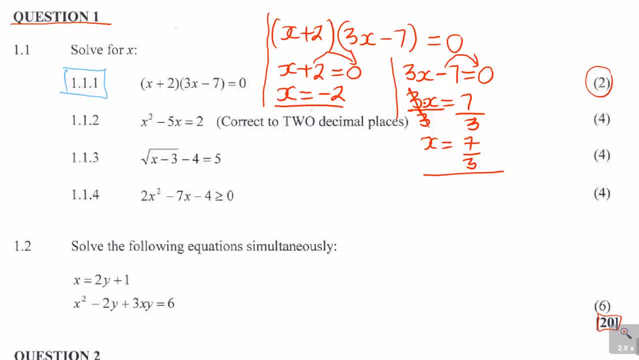 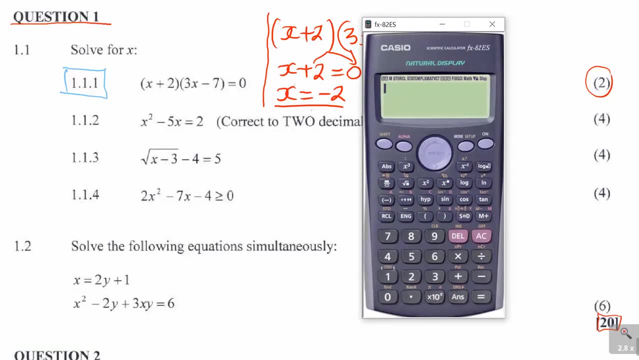 as you said, it's X plus one. I mean X plus two, And you're also given this part of three: X minus seven. So the first value set X is minus two. So you open those brackets where there is X, you put minus two, so it's minus two plus two, And then I've got three. 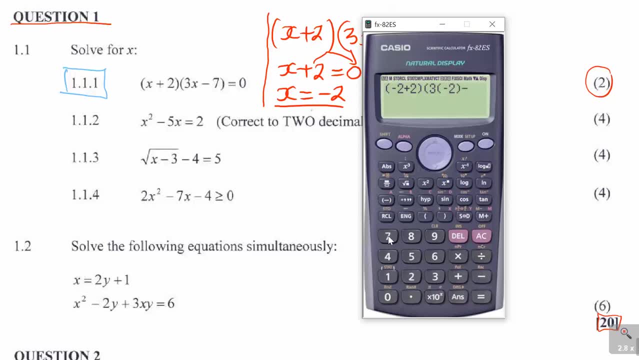 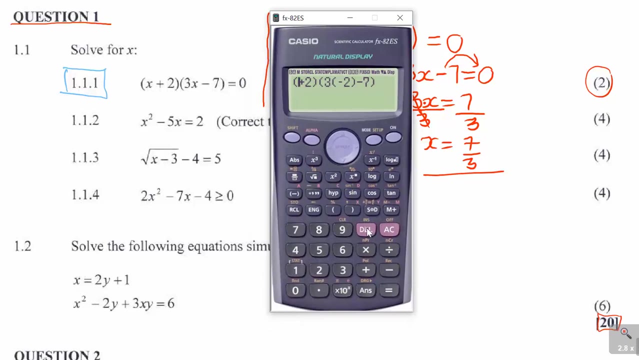 bracket: negative: two minus seven. this must give me a zero, if it is correct. So I'm getting the zero. as you can see now, the other value of x was positive: three over seven. So where there is that I put a bracket of three, or I mean seven over three, not three over seven. 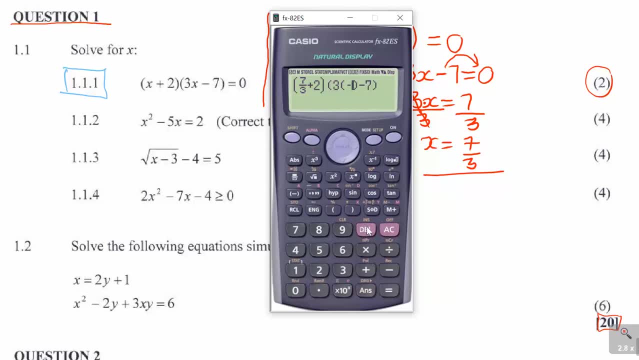 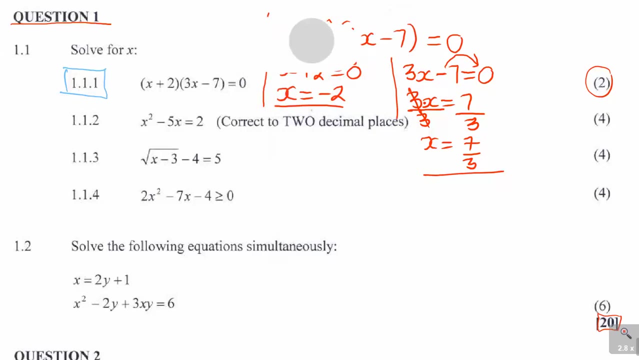 And on the other side again, whether you are negative two, now it would be seven over three. So when I use this value it must give me a zero. you can see equal to zero. So that means says My answer is correct. So that is the first. 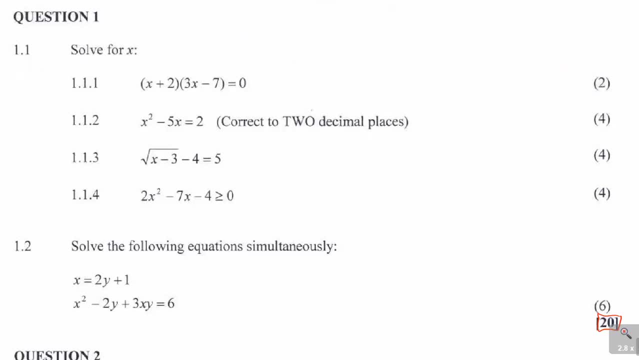 question. question one, point 1.1.. Now we're looking at the next question, which is one point 1.2.. Now he says: You are given that x minus 5x, x squared minus five, x is called to two, And then 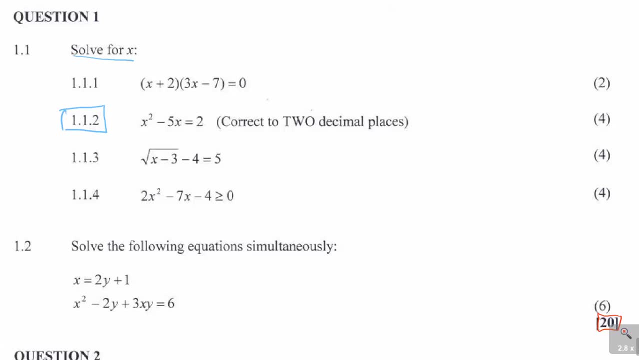 remember where I supposed to solve for x. then there is the key. it says: correct to two decimal places. the moment they give you a question and they say you must round off your answers to two decimal places, remember the approach to that question is the quadratic formula. so now, what is the quadratic formula? 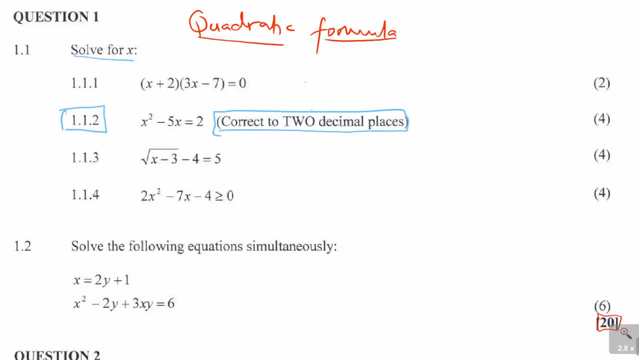 you need to know how to write this formula. as i said, you need to practice well with the formula. so first of all, let us look at this equation. this equation is: x squared minus 5x is equal to 2. but now you need to write this equation in a quadratic general, the general equation of a quadratic. 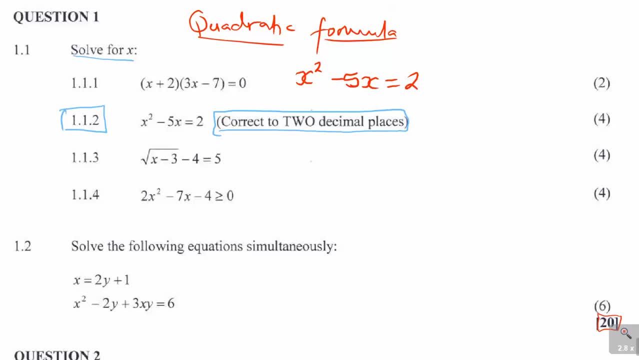 form. now the general equation for the quadratic form is a x squared. okay, you can just do that. so the general form there for the quadratic equation is: a x squared plus bx plus c is equal to 0.. that's the general form of a quadratic equation. so now you need then. 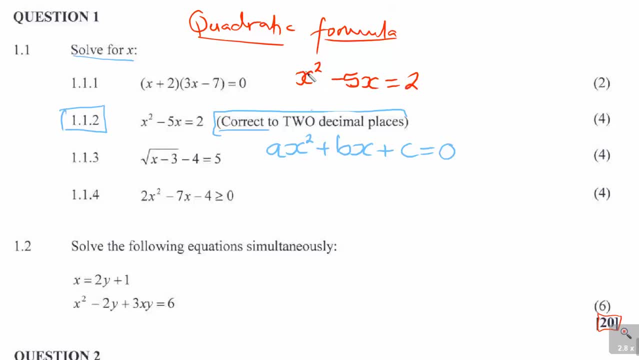 to write this particular equation. as you can see, they gave you x squared minus 5x is equal to 2.. it is not given in the general form. so first things first, take the negative 2 to join the other side, such that you will have x squared minus 5x. now 2 was positive, it will become negative 2. 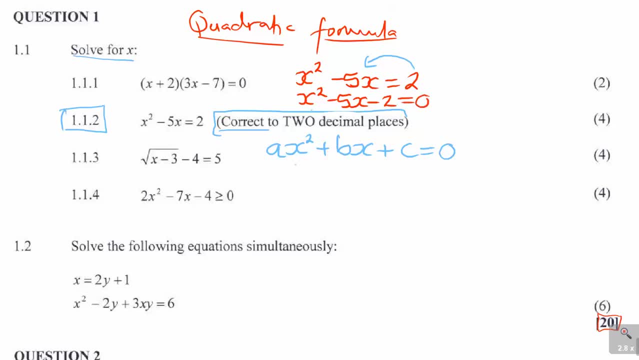 or minus 2 is equal to 0.. so when i write it down here, i will have x squared minus 5x minus 2 is equal to 0.. so you can see that it is now matching my general equation. and because it is matching the general equation, i need to find my a, my b and c. 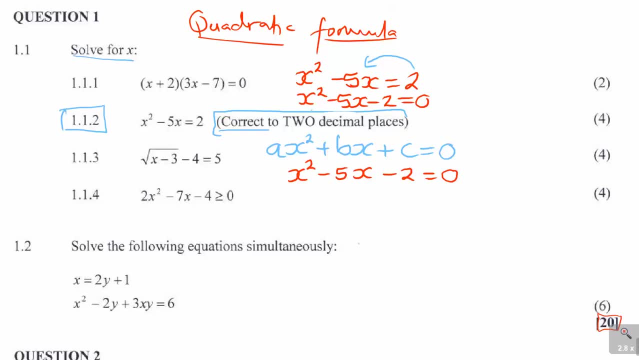 why am i saying that? remember the quadratic equation is given by saying x is equal to minus b. that's the formula you need to know: plus or minus square root of b squared minus 4 ac, all over 2 a. so this is the formula that you need to know by heart, remember. 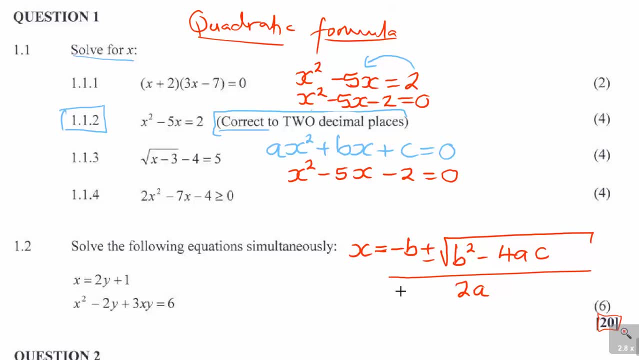 now key things: the division line, this particular division line here that you're seeing. this division line, it must also overlap in minus b. don't write it like this, whereby the division line is only affecting that square root sign. remember, it must also overlap the b part, so be. 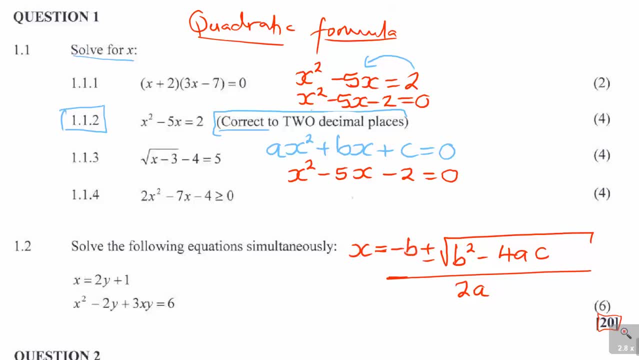 careful about that. that's where sometimes students get it wrong. so, which means we need then to find what is our a, we need to find what is our b and then we need to find what is our c from the formula. so now, as you can see, i have got um the the general form, and i have matched the original. 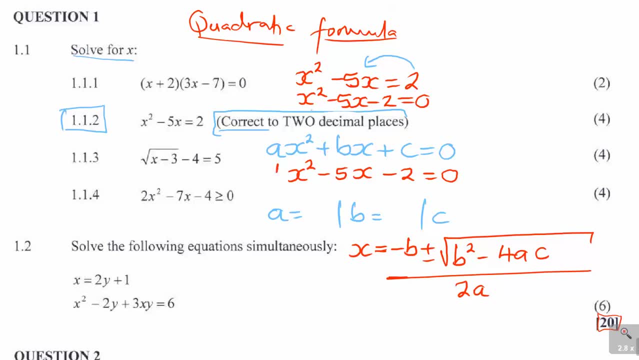 equation. now, if it's x squared, it means that number there. if there is no number, just know that there is a one, so it's one x squared. why am i doing that? if i cut it here like that, you see, it gives me you a and one. if i also cut it here, this we call x squared and in a x squared and one x squared. 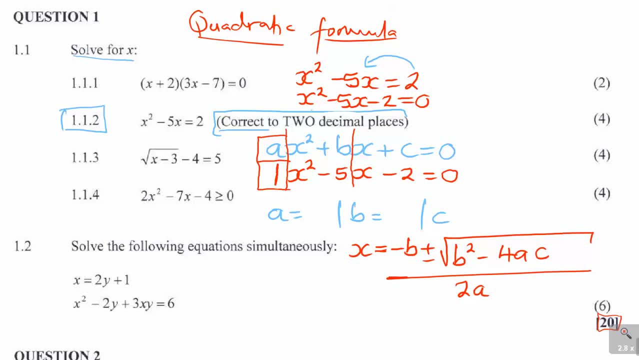 we call a the coefficient of x squared, and which means one is the coefficient of x squared in the sub, in the other one. so in bx b is the coefficient of x, and then we've got minus five. x minus five is the coefficient of x, and then after that one, if i cut it like this: 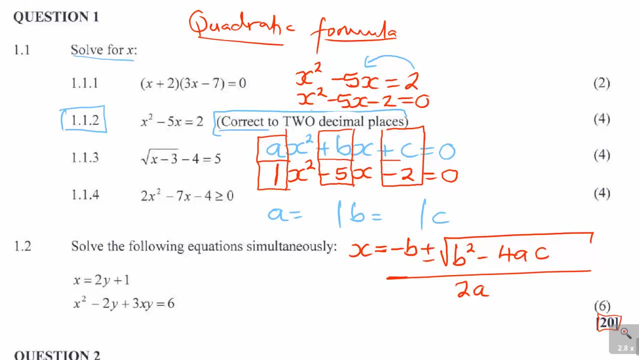 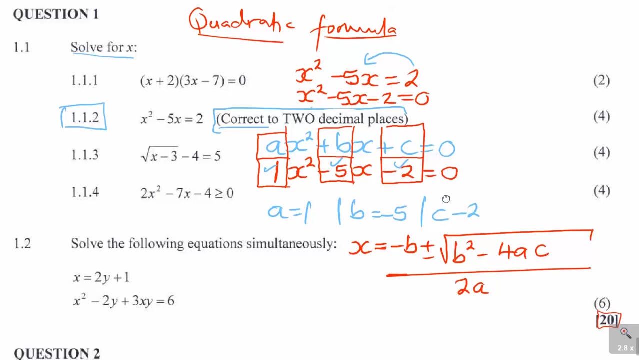 it gives me this minus five. so in a x squared and then one, you can see that my a is a plus five. so my a will be equal to my x squared. but i also need to remember what i'm just doing so that it will help you to identify. you can see now: my a is that which is one, my b is 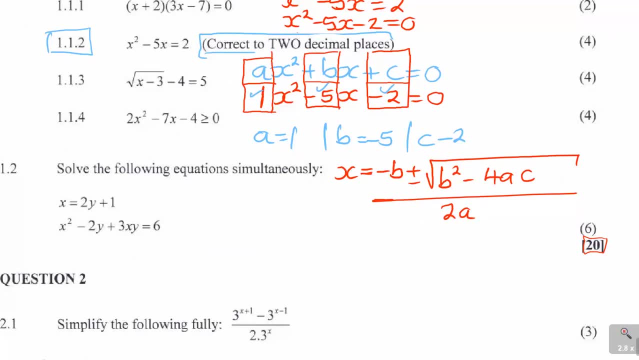 that which is minus five. my c is that which is negative two. don't also forget that the signs are very, very important whenever you're solving this. so now, if i write now in my uh b, remember i must put minus five. so now look at this: the formula has a negative first and 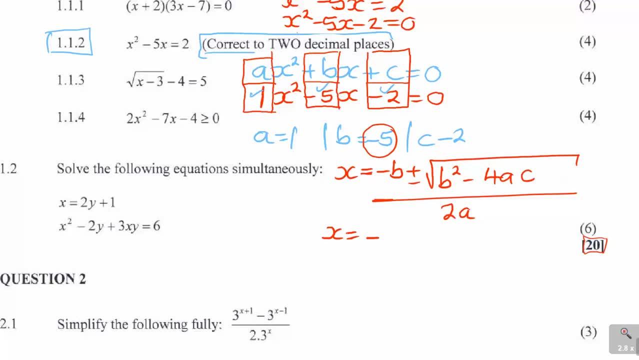 b is also has has its own negative. so you say negative, negative five. so you see how the- uh, they are trying to confuse you there. there are two negatives that you have to deal with: the negative of the formula and the negative of the the equation. so be careful of that. but the 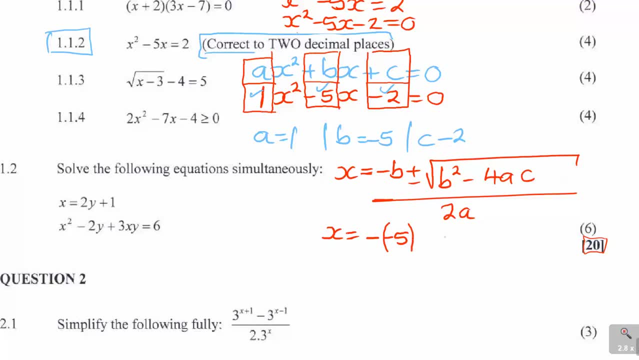 proper way to do it is to put a bracket like that whenever you're dealing with that. but even if you don't put a bracket, the calculator will give you the answer. then you say: plus or minus square root of b squared. again, put a bracket. it's very important now to put a bracket which is minus. 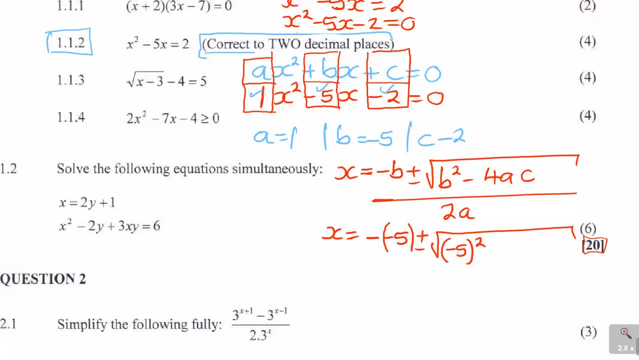 5 squared. if you don't put a bracket where it says b squared, you'll get it wrong. for example, if you write it like this: remember, this is a revision, so i'm trying to show you where errors are most common: if you say where there is b, you say minus 5 and then you say squared, like that. this is wrong, don't forget that. 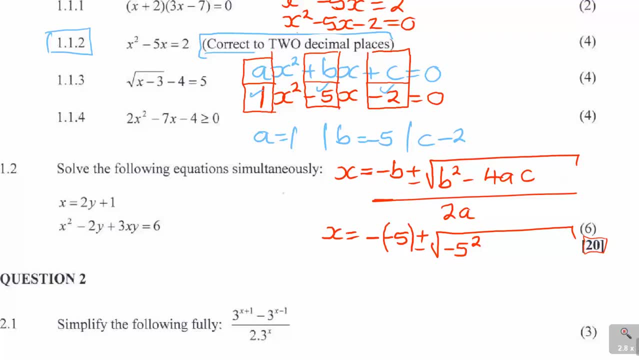 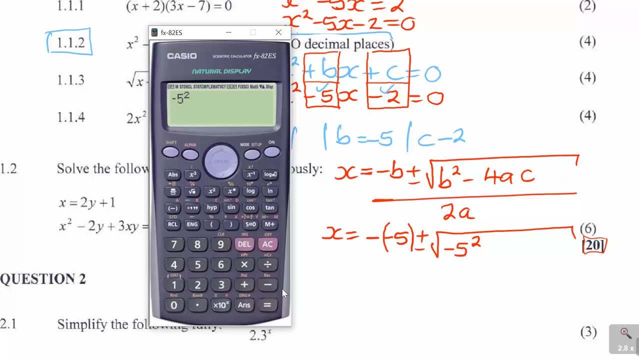 it is not acceptable why. let me show you with the calculator whenever you punch it. with the calculator, if you say minus 5 squared in as much as yes, you put the square, but the calculator interprets that as minus 25. but look if i put a bracket there and if i put a bracket there instead. 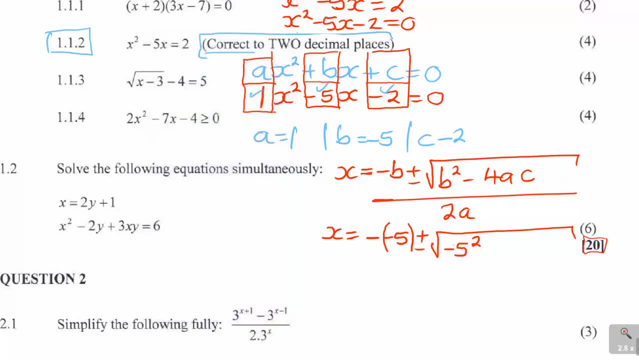 of minus 25, i'm now getting a positive 25, so be careful about that. that's why this bracket inside is very, very important. so we'll have minus 5 squared minus 4. our a is 1 there, so i'll have 1, and then my c is minus 2, so i'll have 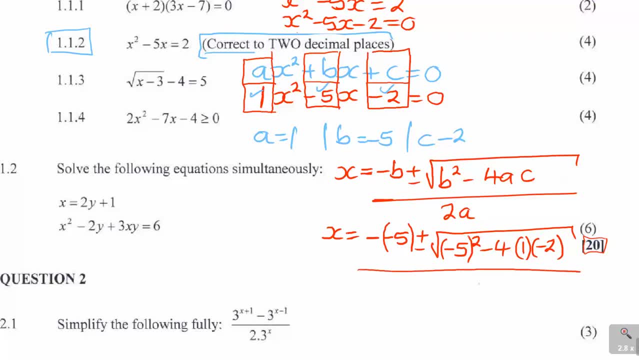 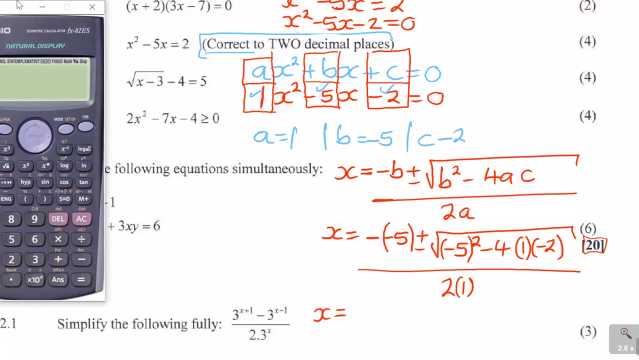 them minus 2, and then everything you're dividing by 2. a again, my a remember is that number one. so you put a bracket one. so always be comfortable to use the brackets. so how do you do that then? as i said, you rely on the calculator to calculate for you. don't try to simplify it, just uh, go to the. 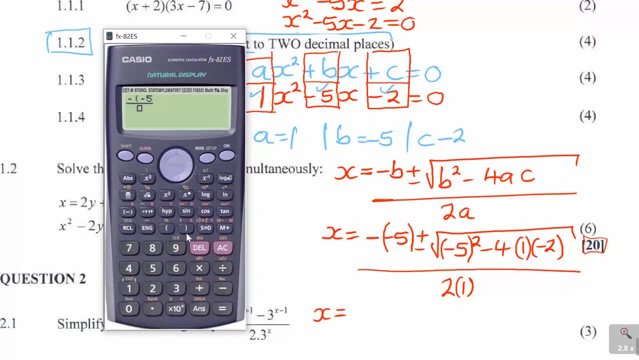 answer straight away. so it's minus bracket minus five, and then you start with the plus square root of bracket minus five. squared minus four, my a is one and my b is minus one, and then you start with: my c is negative 2. you see that, and then you divide by 2 bracket 1. don't forget that if you. 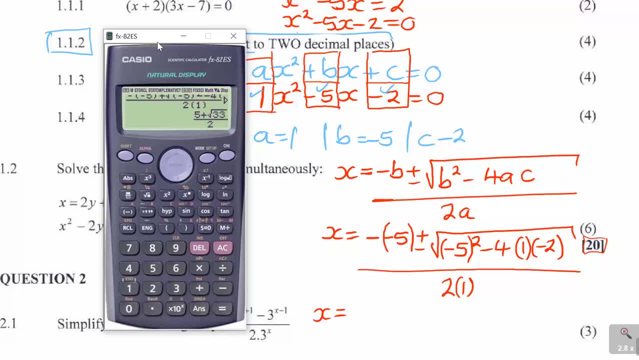 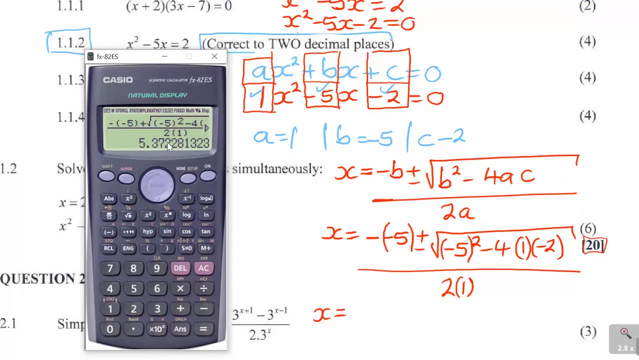 can do this, you won't get it wrong. remember they say to two decimal places. so you press sd and you can see the answer is 5 comma 3, 7, 2, 2, 2. so in two decimal places is 5 comma 3, 7. you need. 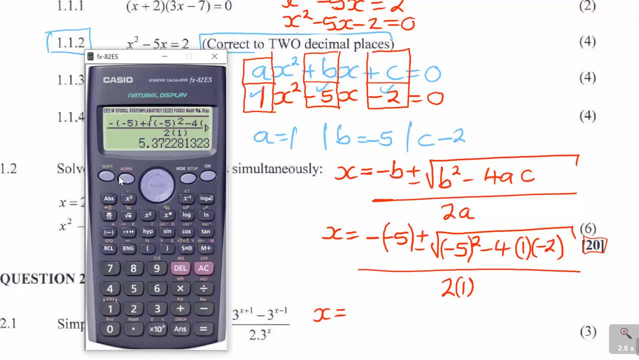 to know how to round off. but your calculator can do it for you. what you do? you say shift, set up, and then you look for 6 where it says fix. so you say 6 now by fixing, is asking you up to what decimals must be, must be round it off for you. so the question: say two decimal places. so 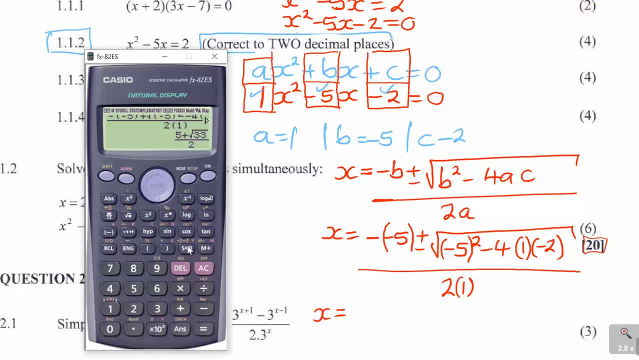 you also fix it in two. when you do that now, when you press sd, do you see that you are getting now the answer, which is 5 comma 3, 7? now i need to find both answers because i don't want to punch this again with my calculator. i now remember. 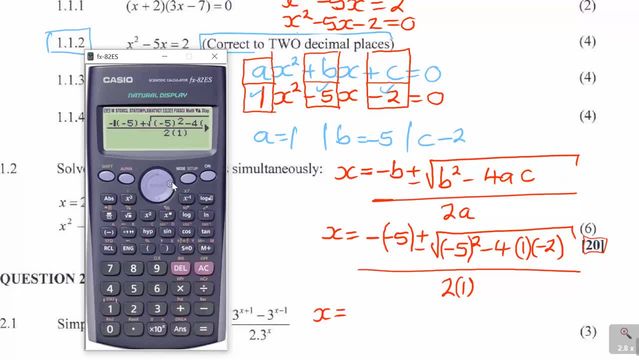 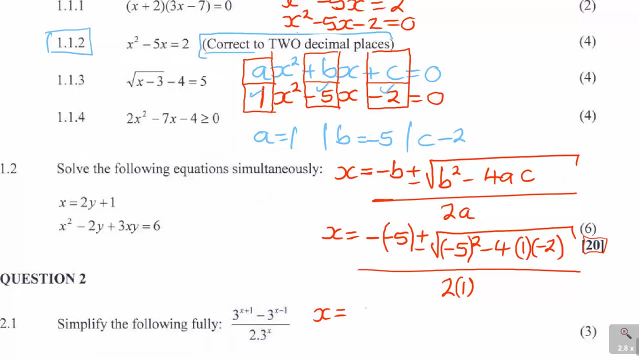 the answer is 5 comma 3, 7. that's the first one. now you delete, put minus. check the second answer: equal to. so from 5 comma 3, 7. the other one is negative: 0 comma 3, 7. so we had 5 comma 3, 7. 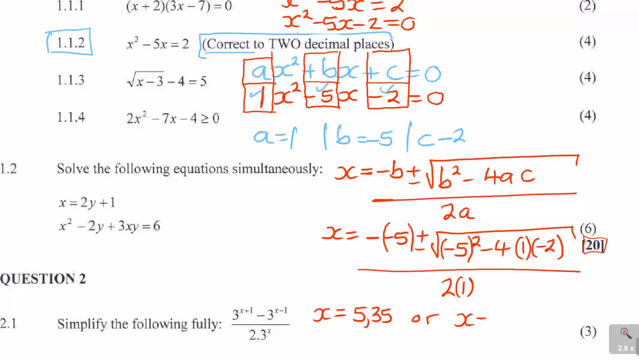 or x is equal to minus 0 comma 3, 7. now remember that these answers are rounded off to two decimal places, according to the requirement of the question. as you can see, they says two decimal places. so that's how you solve this particular question, but 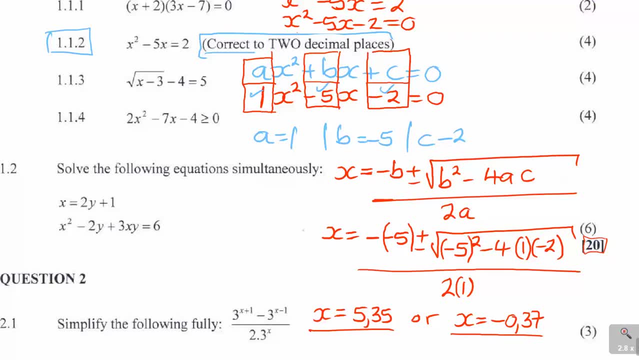 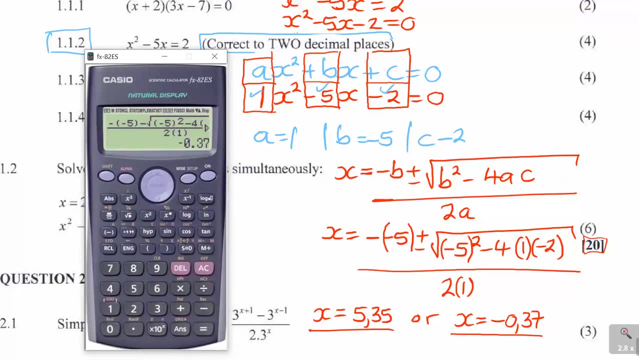 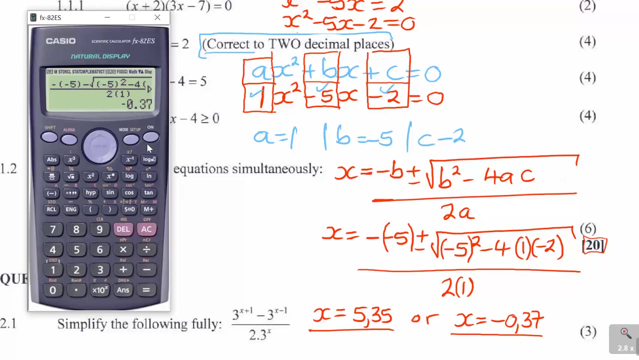 i always encourage students to test your answers. so what you do is you go to one of those, whether 5.37 or negative 0.37. so how do you test that? so for you to test that, remember i've got this answer here, so i'm going to test with the rounded off answer. so test with the original answer for. 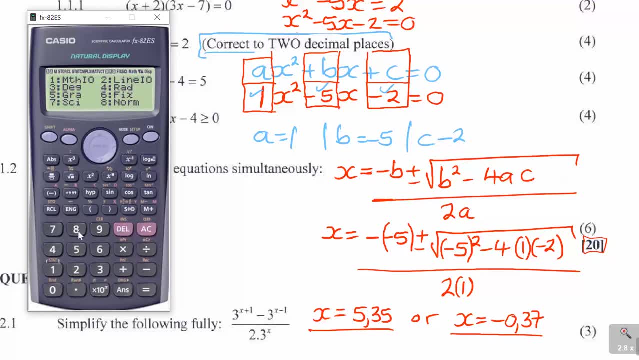 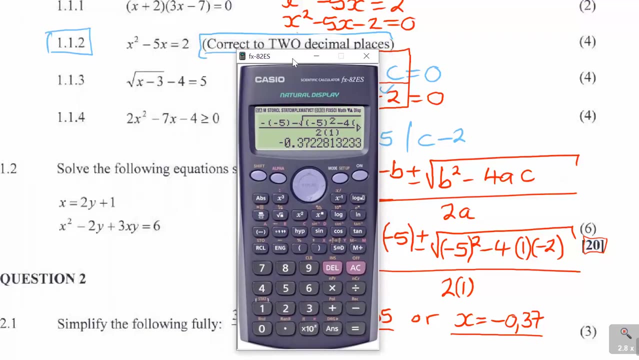 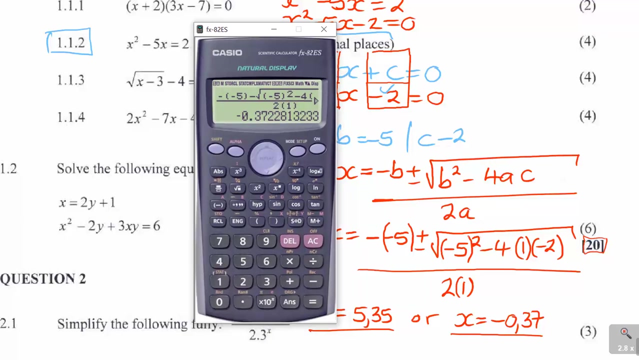 example, if i, if i say shift setup and i take it back to 8 as normal, and say sd, you see it takes back to the number that is not rounded off. i press 8 to return back to normal. so this number, i'm going to use it into my original equation, which was x squared minus 5x is equal to two. so when, whenever, 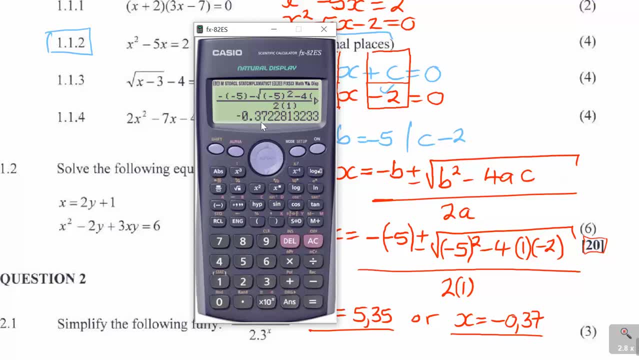 is x. now i put the value negative 0.37. so if i press s ac and then i say answer equal to it gives me that last answer that the calculator was having. so which means if i come to the original and say x squared, where there is x squared, i say answer squared minus 5 answer. remember the answer? 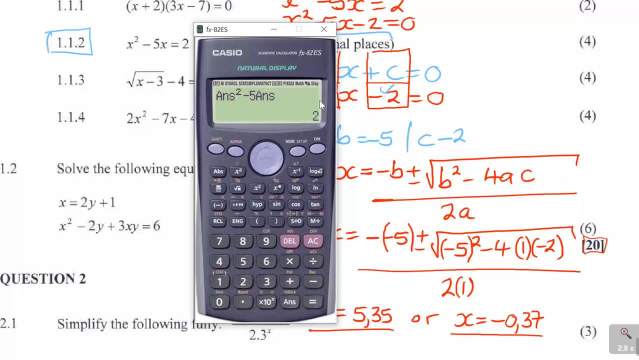 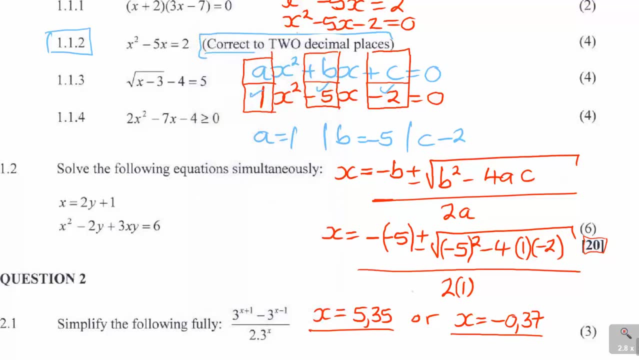 is that particular answer. it must give me a 2 which is equal to 2.. you see that why? because i substituted the original question into that. but if i now try to use my rounded off um, answer now what you'll see with the challenge of the rounded off one. for example, if i use um 5.3- uh, let me just see this one. if i 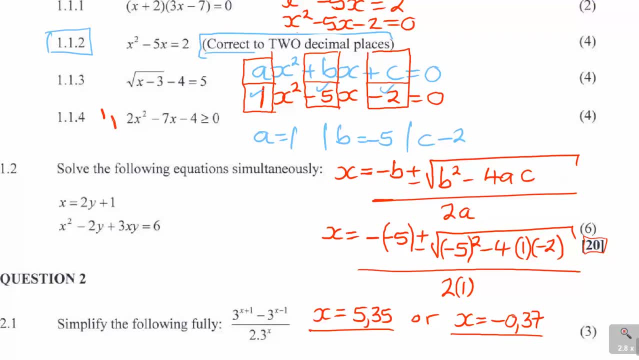 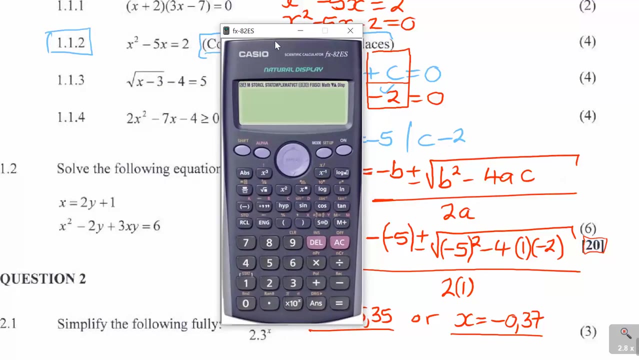 say five comma three five, and i'm, if i'm going to use 5.35 in this particular case, um, it might not give me, uh, the answer of two. you know why? because it is rounded off. so, for example, if i use, instead of five comma, listen, let me use minus zero comma three seven, like previously, is negative zero. 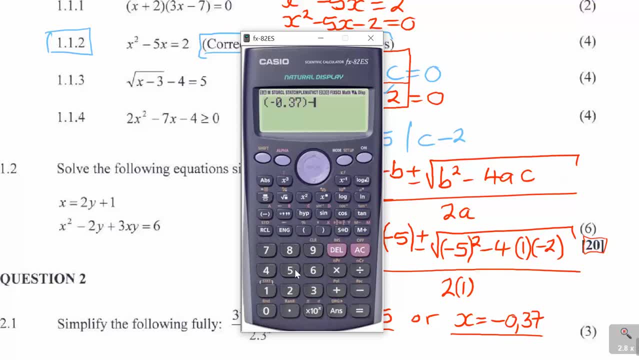 comma three seven, squared minus five, bracket negative: zero: comma three, seven. remember the first one did work. but look at this: if i press sd i'm getting one comma four, eight. you know, i know, one comma four, eight is actually. did i square that? okay? no, i didn't square that. it must be squared. all right, it gives me one comma nine, eight, six, nine. 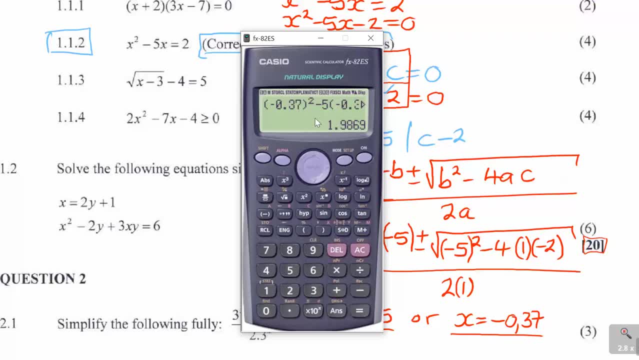 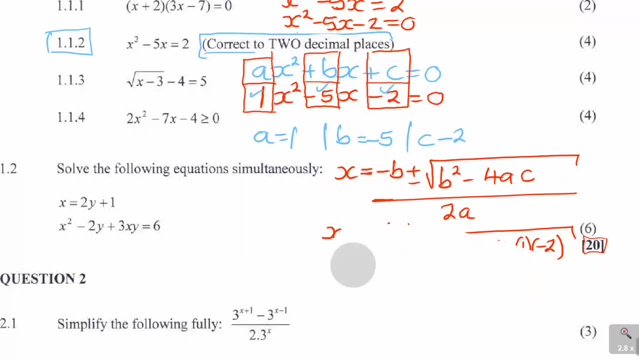 now rounded off, it becomes almost two, which is fine, but you can see that it's not the exact number that i got, but that is how you can work on that problem, so it is the solution to that. now let us look at the next one. the next one is question uh. 1.1.3 says: 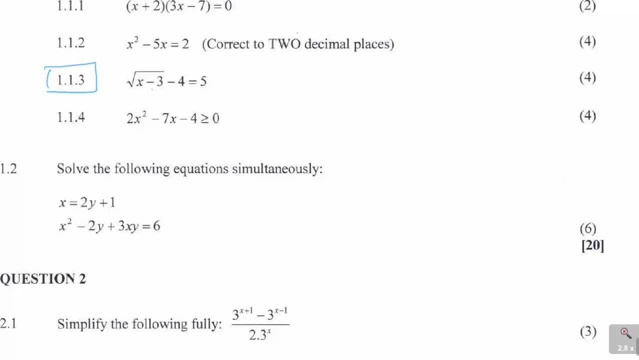 what is the solution to the problem we have to solve for x? so if we are supposed to solve for x and they've given you that x square root of x minus three minus four is equal to, it's called to five. now this is the solution that you need to work for. 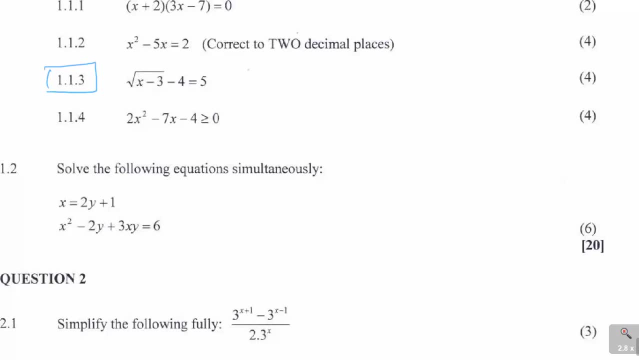 when you're dealing with um roots. these are roots. so what you need to do, first things: first, you need to identify that this part x minus three and then minus four is equal to five. you need to understand, understand that the negative 4 is not affected by the square root, so the minus 4 must be transposed. 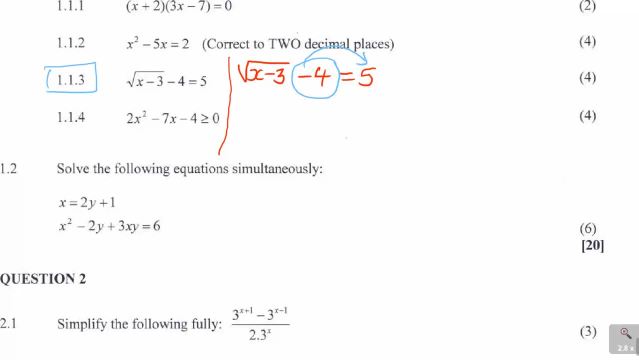 to the other side before you can do anything with the square root. Remember, I know that. you know with the square root you have to square, but you cannot square when that 4 is still there. So you need first to take 4 to the other side so that you only have the square root on one side. So you will. 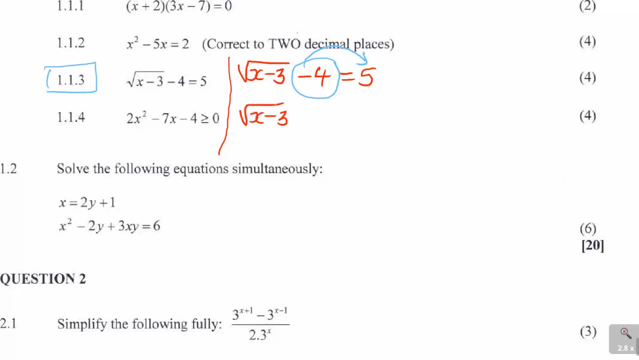 have square root of x minus 3, so on this side is equal to 5.. Now the negative 4 will become plus 4.. That is the first important thing you need to do, such that you've got x minus 3 is equal to 9.. 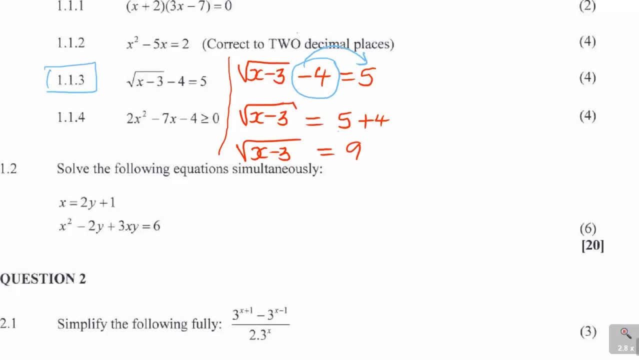 So don't forget that first of all, you need to do whereby you take everything to the other side. Then, when you have done that, you can then get rid of the square root. Remember, you put a bracket and you square, But what you do on the left, you also do on the right. That is how you get rid of that square. 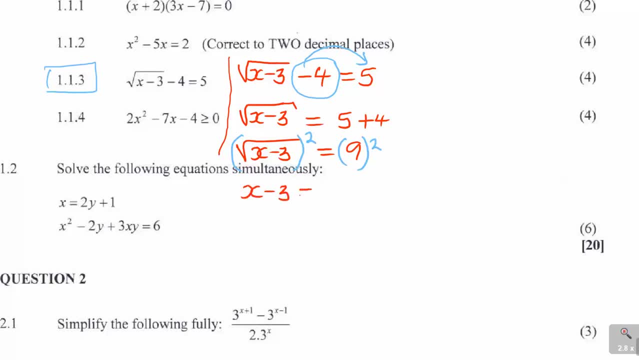 root. Then you will have now. x minus 3 is equal to 9 squared. I can maintain it as 9 squared is fine, or you can change it to 81.. Then take minus 3 to the other side. You will have. therefore, x is equal. 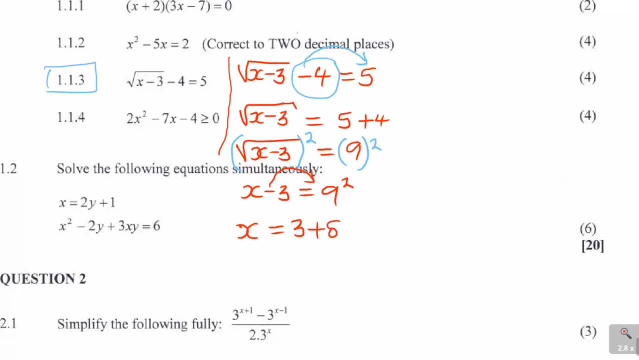 to from negative 3 is 3 plus 81 and therefore x is equal to 84.. So you see, that is the first important thing you need to do Now. the negative 4 is not affected by the square root, but it is the value of x. in this particular case, You need to test it Where there is this. 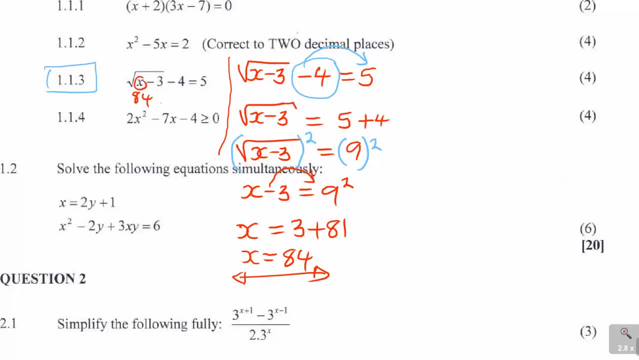 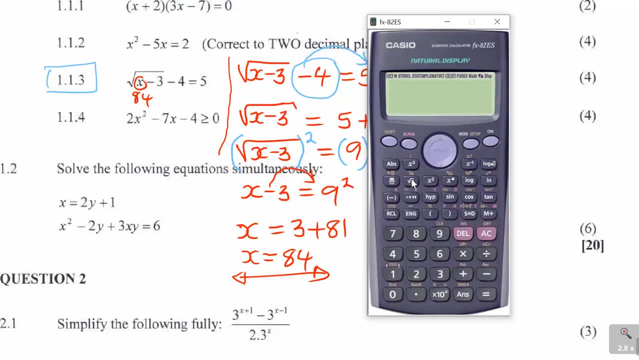 particular x, you are going to have what 84. So let's test that and see what answer it will give us. It must give us 5 if we put 84. So square root of 84 minus 3, then play forward and say minus 4. 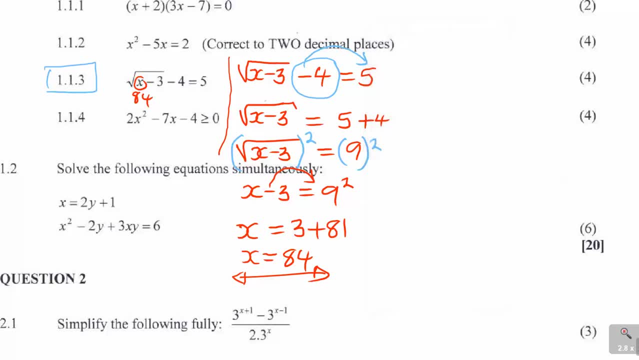 because it's not under the square root. You see, it's giving me a 5, which is correct. So that is how you can approach the square root of 84.. So that is how you can approach the square root of 84.. This particular inequality, and I hope this is making sense, And you guys, by the way, before I, 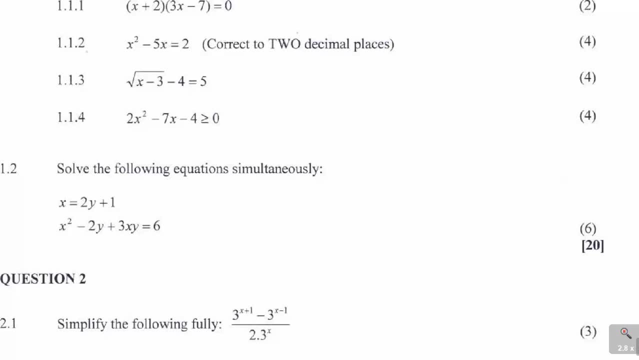 forget, if you have not subscribed to our channel and it's the first time to see our channel, I will encourage you to subscribe to the channel so that you can get notifications every time we post a new video, Also to be notified in real time when there is a video that has been uploaded, you can 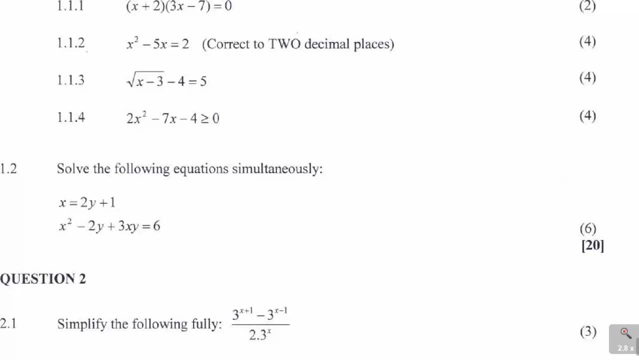 also make sure that you switch on that notification bell. There is a bell in front where you can press it. Now, what it means is, every time there is a new video, immediately it is uploaded, you guys are able to also get a notification from YouTube. All right now, continuing with this. 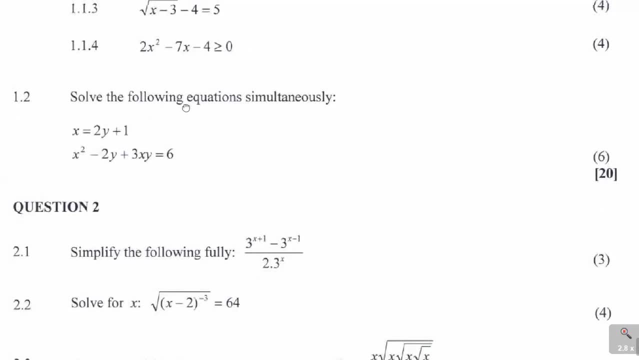 other one that was 1.1.4.. So you can see, these are good marks that you can get advantage of in your final exam. So what are we looking at here? It says: 2x squared minus 7x minus 4 is greater than or equal to 0.. 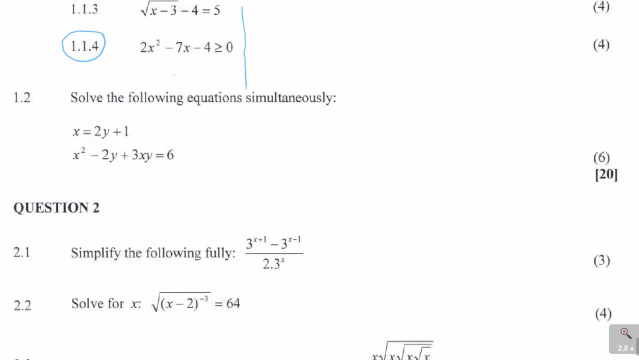 These are inequalities and it's very, very important for you to understand how to solve them. So what we have is 2x squared minus 7x minus 4 is greater than or equal to 0.. I know there are many ways of factorizing this again, but I will encourage you if you're already. 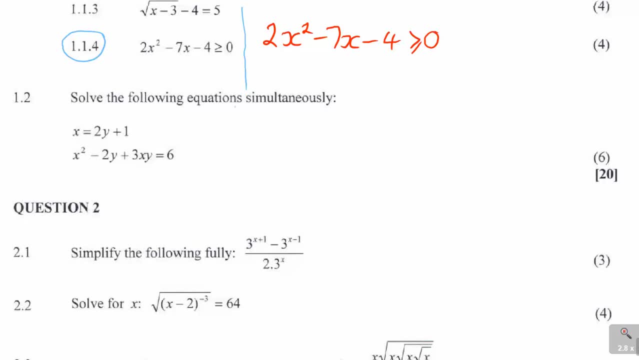 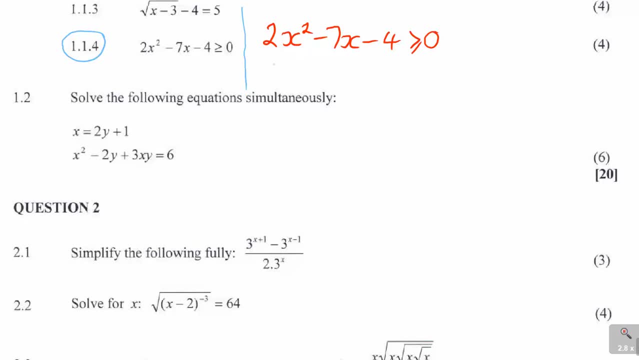 get your answers. Remember, the general form says: ax squared plus bx plus c is equal to 0.. So what you do in this particular question: first remove that sign and instead of the sign, you change it into an equal sign. Remember, don't forget, that you must first change that greater than or equal to. 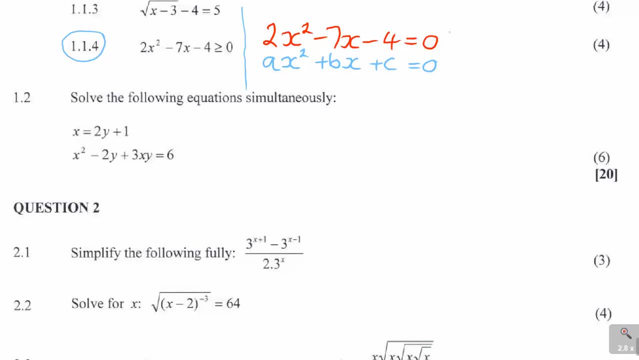 0.. So you exclude the material you have changed into an equal sign and then find the same thing. So I basically give you the example where x is equal to 10 over 10.. And of course, if you think you have to change something like right or left or right, or left or right or right or 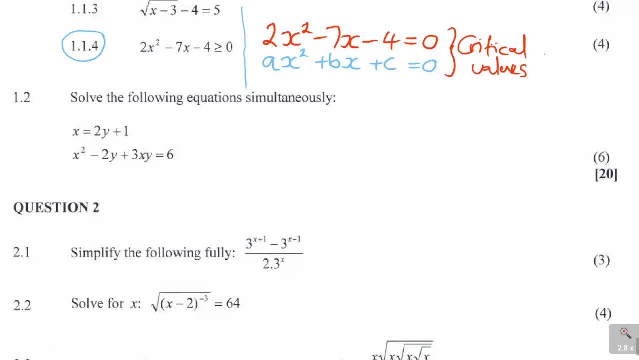 left or right. you can then also just cut what we have, y. So the cosine of what you did is you cut away away this middle point of e in. we think that you have x equal to 10 over 10 you. that is why I'm doing that. 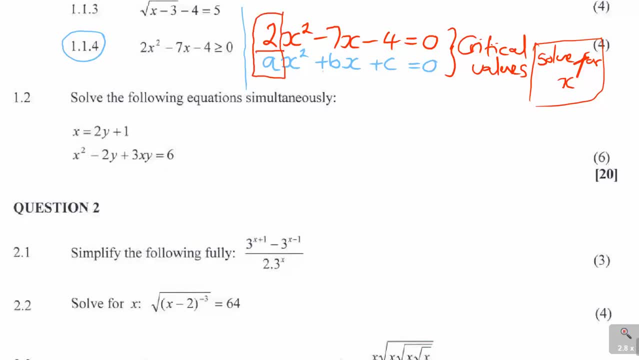 So that is why I am doing that. So in this case, something can be changed in this situation and we need to solve equation 点. the coefficient of x squared there is 2, so a is 2 there, a is equal to 2. you cut before the. 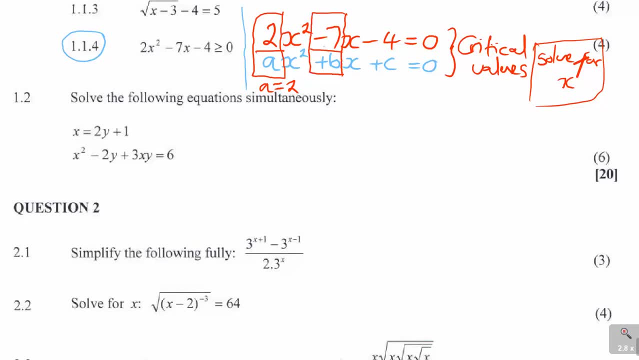 coefficient of x, you can see b. b is that number, so b is equal to minus 7. and you also cut like that you can see c is that number which is minus 4.. so that's what you're having. then you write the quadratic formula. it says: x is equal to plus or minus square root of b squared. 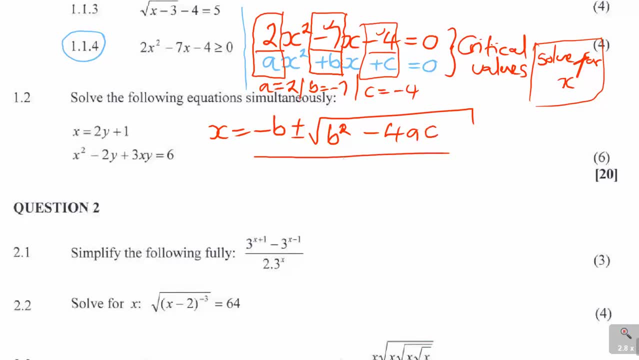 minus 4ac and everything is divided by 2a. so now you conclude and say x is equal to minus. remember b is negative 7. so there is the negative sign of the formula, like we did previously. and now we are saying minus b is equal to minus. remember b is negative 7. so there is the negative side of the formula, like we did previously. and 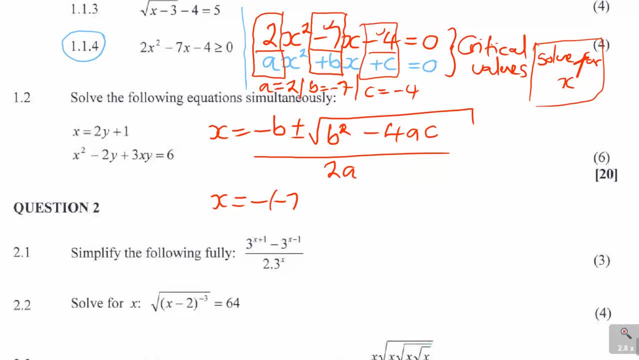 the negative 7 there. but it's good to protect that with a bracket plus or minus square root of b squared. put a bracket and say minus 7 squared minus 4. my a is 2 there and my c is negative 4 and this thing is all divided by 2 and my a is a 2.. so it will give us two values of x. 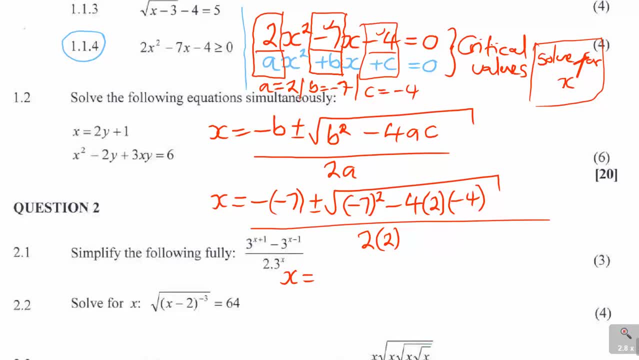 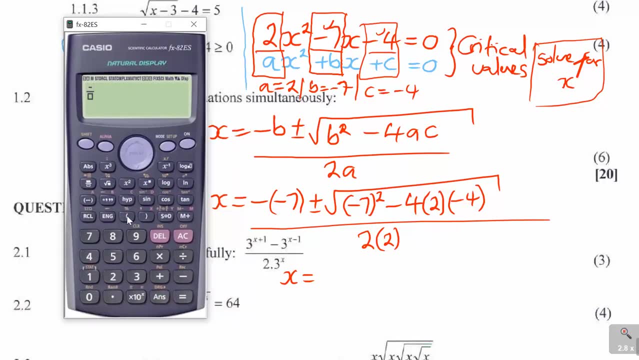 which we call them the critical values. so when you do that, you will have um negative bracket, negative 7. we start with a positive plus square root of bracket negative 7 squared minus 4. my a is 2 and my c is negative 4 and this is all over 2 into 2, so that's. 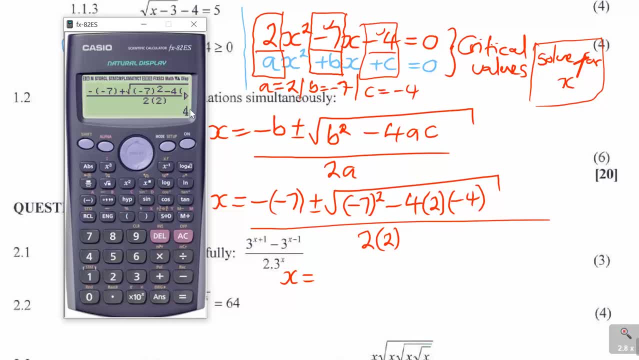 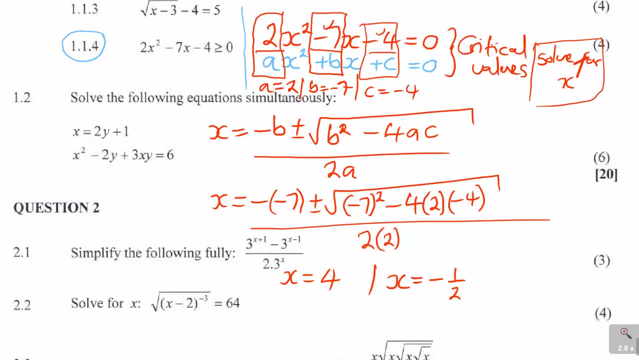 what we have and you can see. the first answer is x is equal to 4, and then we play back with the negative. so x is equal to 4 and x is equal to negative half. so those are called critical values, just as we talked about. say, you are solving for the what for the critical values. 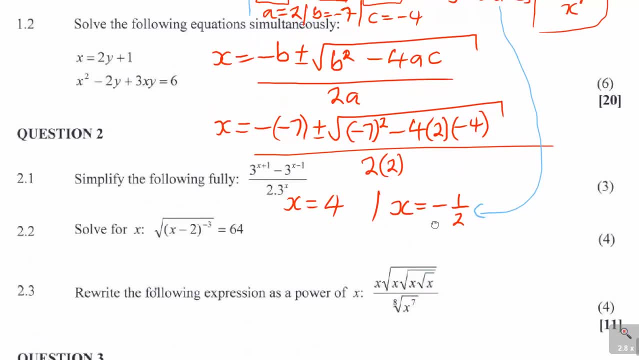 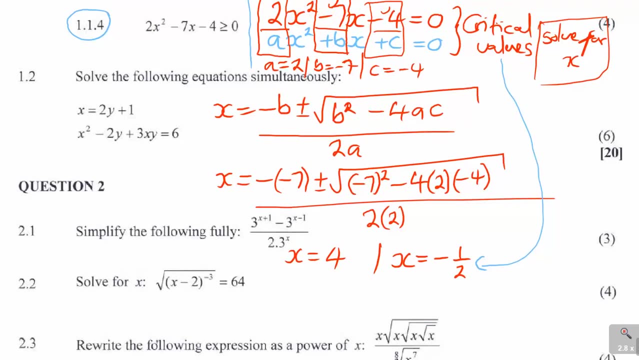 now, when you get the critical values, now you need to come back to the solution to say: why were we doing all these critical values? so what you do is you have your number line with the critical values like this: all right, and then remember your critical values is x is equal to you. start with. 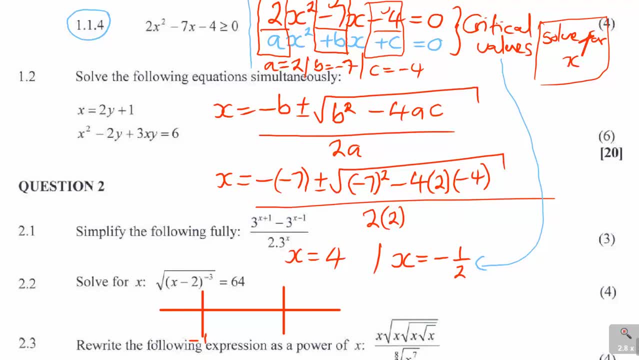 negative one, negative one, or you can say negative zero, comma five you, because that is the half and then the other one is four. that's what you're having there and you start testing the values. so what you do is you go to your original here and don't worry with the sign. you're just looking at the before the sign there and you're going to 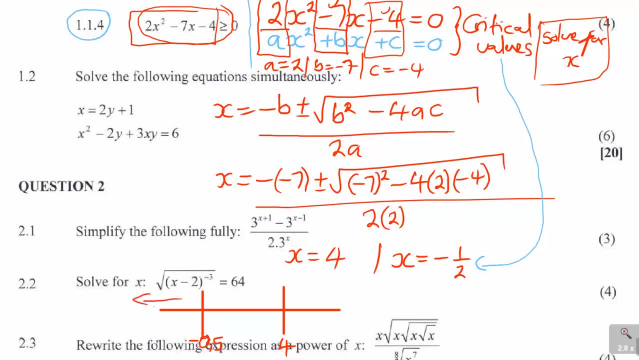 test, for example, you look at a number before zero comma five, choose any number like minus four. so you take a look at the number before zero comma five and you look at the number before zero comma five. it's like a calculator and what you do is, whether it's x, you put that particular value. so if you're choosing any value, 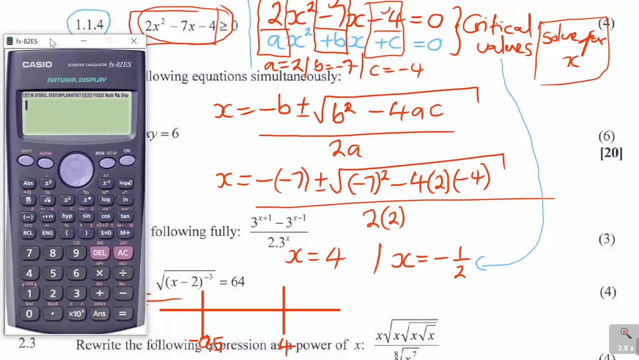 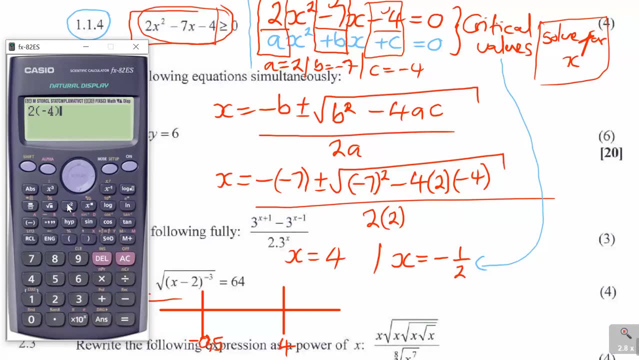 that you think of you can just just use in this case. so, for example, I use minus four, so two bracket, I've got negative four squared. just any value AFTER zero comma negative. zero comma five minus seven, bracket negative four and then minus four, is that the previous one negative one. so any absence of a slash negative one will give you a 마리. will give you a syringe which would stay until you get to number 4. this might be a very careful step that you put in place your previous equations, you know. so what you do is you simply put this into a calculator so you can just activate, like this row, this row, nephew two, and then you calculate here: how are we doing so you can justический the cells in here. 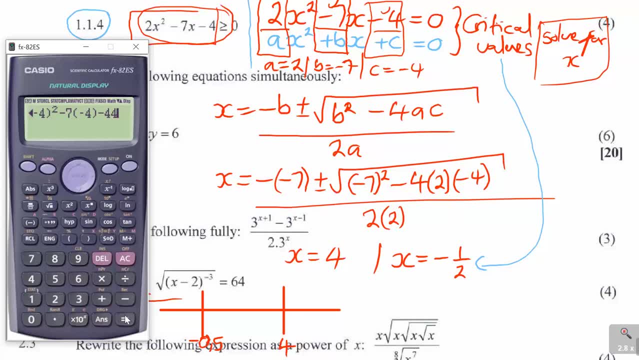 out and then you get your whole village square. you can classify them so you can calculate this. when you do that, it will give you um the answer and you can see i'm getting 56. but don't worry with the answer. you focus on the sign. 56 means it's positive. now choose another value which is: 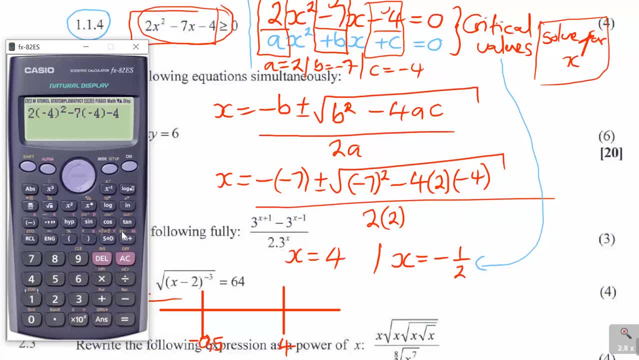 between negative 0.5 and 4.. like we can choose a value like 3, because 3 is just before 4, i can choose three, but zero is the simplest one that you can use. so if i choose three, you see the number changes to negative. so i had a positive, now it's a negative. let's choose a number after four. 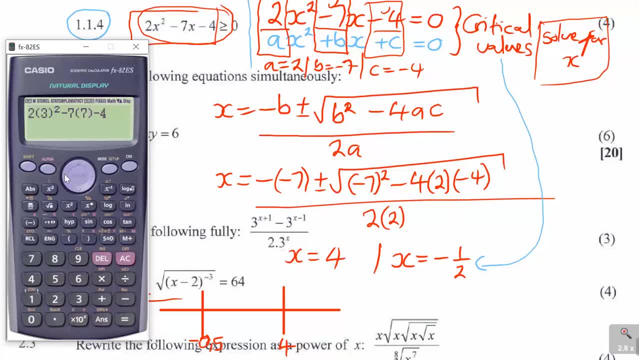 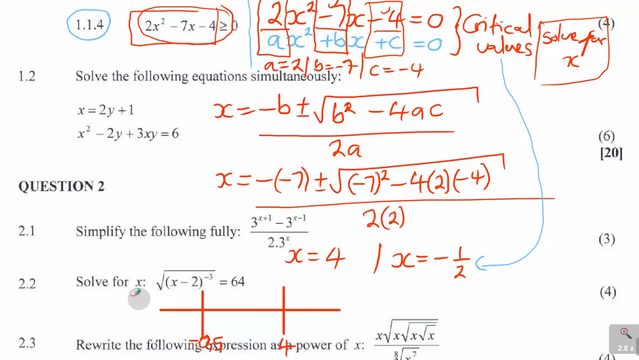 it can be seven. so remember i got a negative, uh, in the other one. then now i put a seven. now i'm getting a positive again. so the signs where i got a positive, here it was a positive, i got a negative and then i got a positive. now, when i got back to my original, 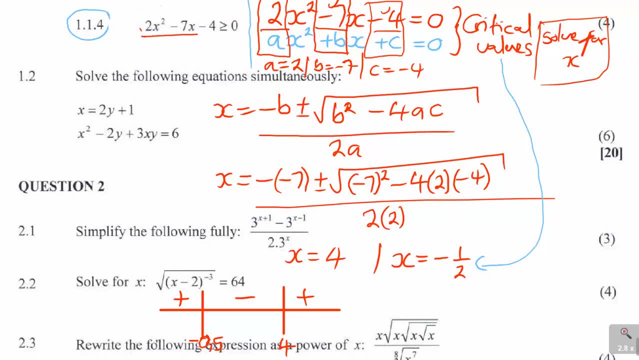 question. the original question says this is greater than or equal to 0 and anything greater than 0, meaning it's positive. don't forget, anything greater than 0 is positive. so it says on my sketch: here i must come and look for the positive signs. so 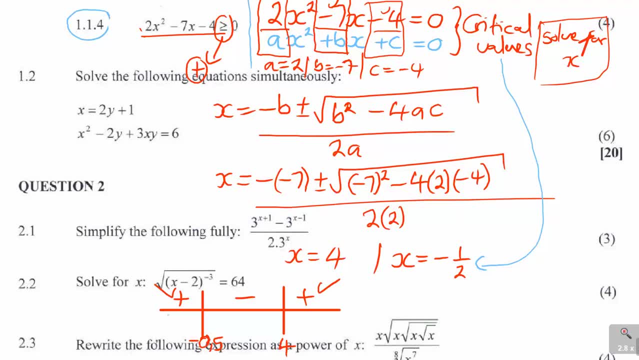 can see, i have a positive on the outside of these values. so how to write them? the first one you can see is going this direction. so it's x, that same direction. but this case is the sign. x is less than the critical value, there is negative 0.5. but now, because they say greater than or equal to you also, 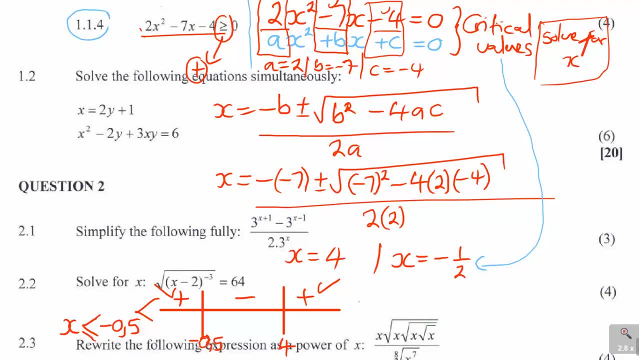 maintain less than or equal to, then the other value is on this direction, which is x is greater than or equal to the critical value, which is that one greater than or equal to 4.. so those are the two values: x is less than or equal to negative 0.5, or x is greater than or equal to 4.. please don't be tempted to say: 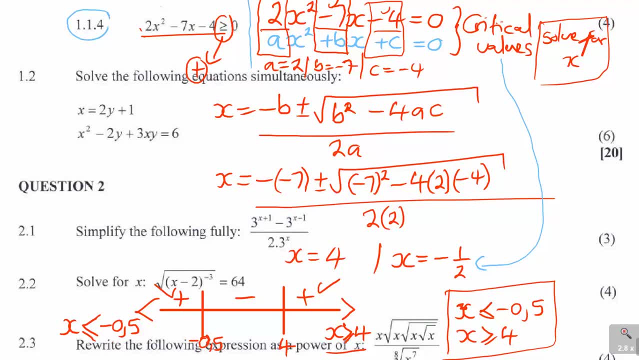 your answers. some students, they just solve for x. after solving for x, they use that sign and they write: x is greater than or equal to negative 0.5 and x is greater than or equal to 4.. you can see that one of them will be correct, but the other one 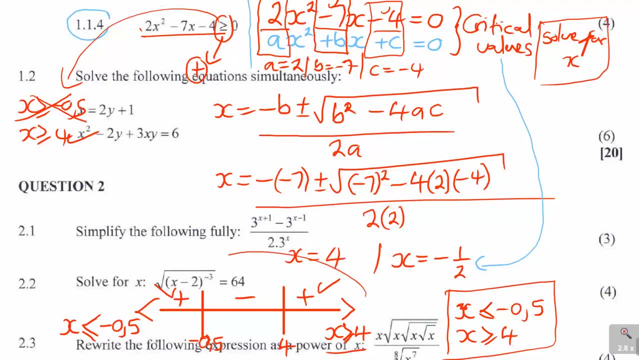 will be wrong and you're going to lose marks again because they are going to mark you that part. if you don't have it, you're going to get out of four mark, you just get one mark. so be careful how you solve that inequality. now, as i said, i hope this guys does give you some- uh, what you call it- some. 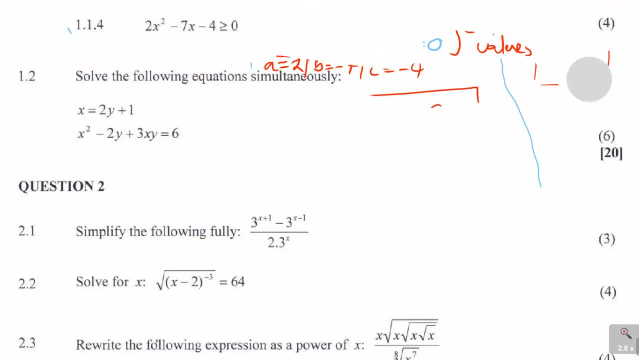 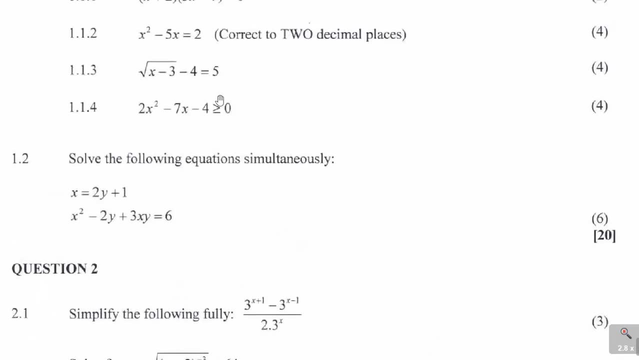 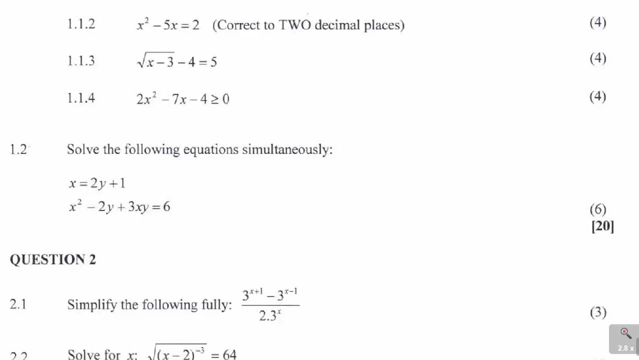 revision of some sort, you are able to learn and see how to solve um for the, what you call. you are able to solve for um, solve for x in this case. the last one is the inequality question 1.2. say solve, i mean the simultaneous, the simultaneous equation, six marks, it's good. 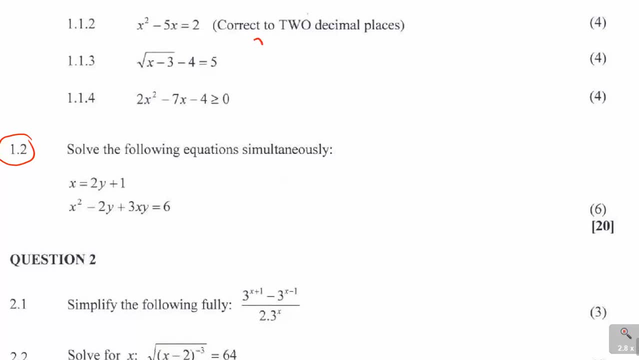 marks. you are solving um. you're given already x is equal to 2y plus one, and then we call this equation one. and then the second equation is: x squared minus 2y plus 3xy is equal to 6, and then we call that equation 2.. so what we're doing is already equation 1 is very simplified because already 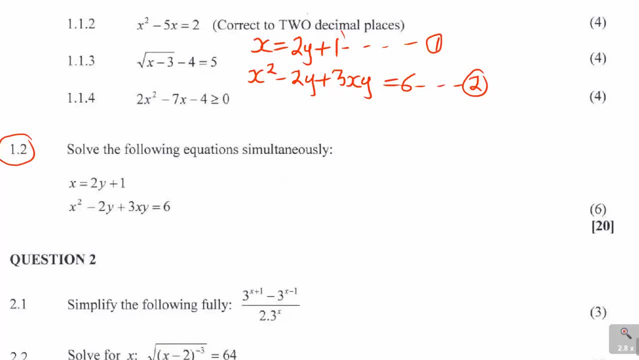 it is given as what is x. so where there is x, we're going to put this value. so where there is x, which is x squared, so u instead of x squared, you say 2y plus 1. that's where it was x previously. that is squared minus 2y plus 3 into 2y plus 1, and then y is equal to 6.. 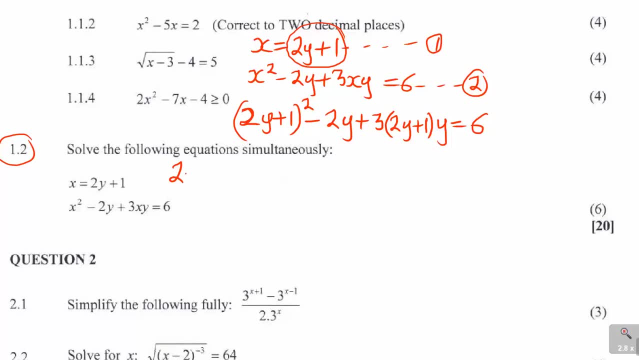 don't forget: 2y plus 1 is 2y plus 1. squared is 2y plus 1 and 2y plus 1.. now students usually say 2y plus 1 is is like this: 2y squared- they forget- is 2y. 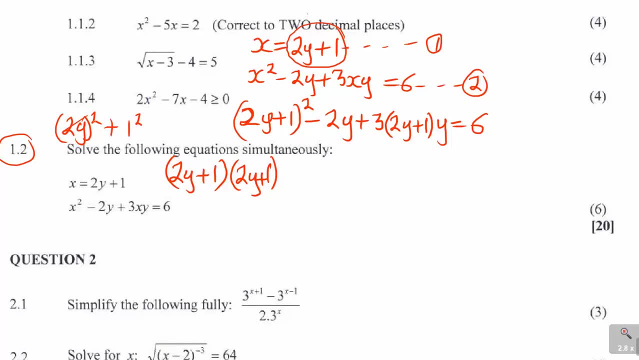 squared plus 1 squared. that is wrong because you need to expand this whereby you're saying 2y times 2y, it's 4y squared. because 2 times 2 is 4y times y, it's y squared 2y times 1. 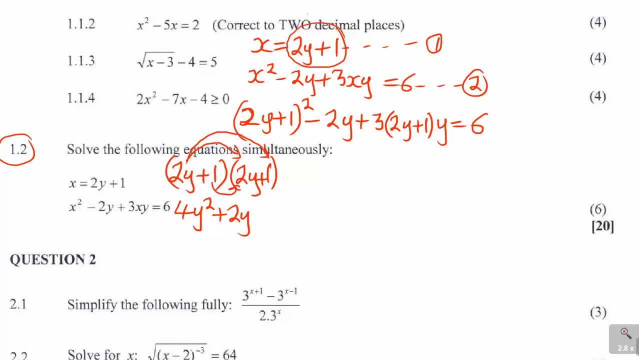 it's plus 2y, then the other one, 1 times 2y, is plus 2y. so we are expanding the normal expansion. 1 times 1 is plus 1.. don't forget that. so is that minus 2y, now plus 3.. now this y is good to come. 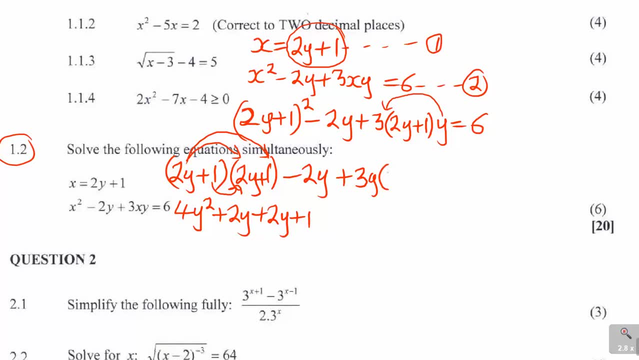 and put it just next to 3, so that it multiplies once 3y 2y plus 1.. then take the 6 back to become negative. 6 is equal to 0.. now the 3y multiplies 3 times 2, so we had that minus 2y, the 3y 3 times 2. 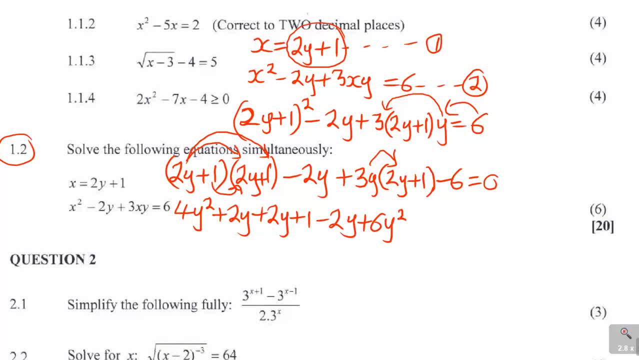 is 6y squared because it's 3y times 2y. 3y times 1 is plus 3y minus 6 is equal to 0.. then collect like terms. for example, there is the 4y squared with 6y squared. 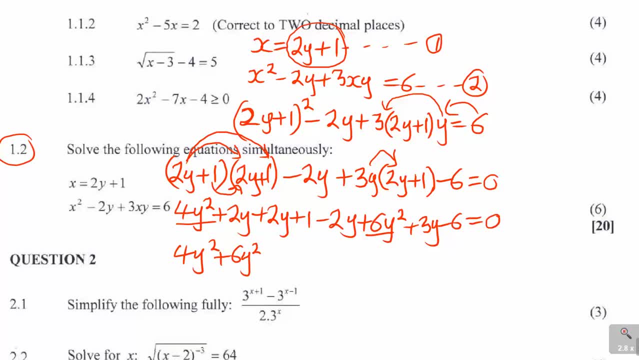 be very careful here. they just want to test, if ever you are able to recognize errors. now let's look at the y. we have 2y, you have 2y. we have minus 2y. we have, uh, positive 3y, so i will have plus. 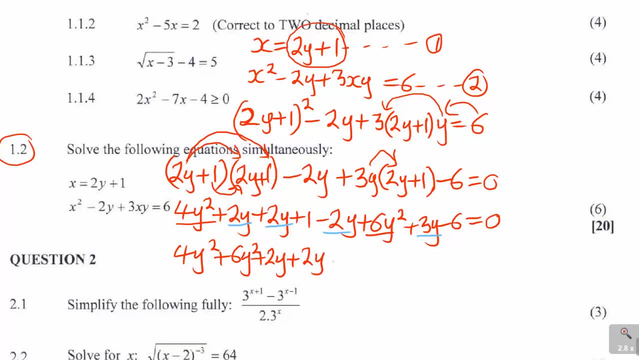 2y plus 2y, minus 2y, and then i have got plus 3y and then the last one i have is a 1 and a negative 6. so which is plus 1 minus 6 is equal to 0. then you go and check: is there any of the items that? 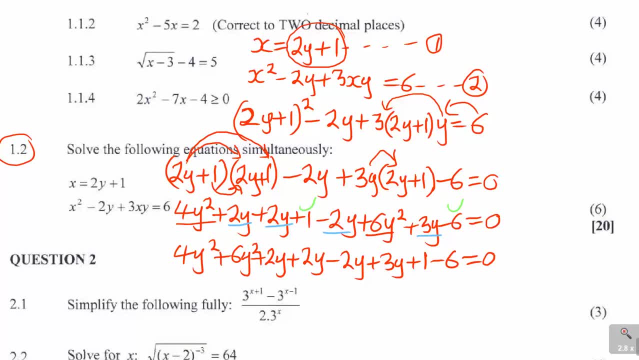 you forgot all of them. just check if it's either ticked or marked. so that is a way to check that you didn't make error. now the next step is 4y squared plus 6y squared. it's 10 y squared, now 2. 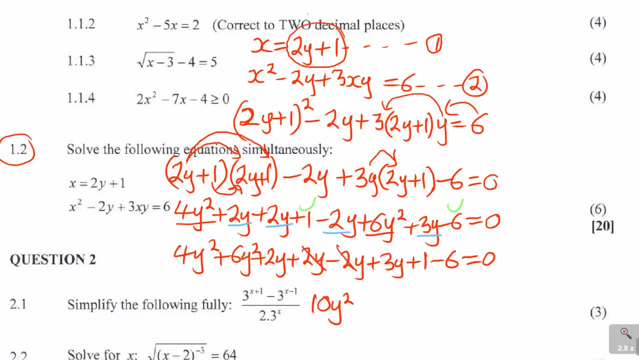 plus 2 minus 2, this goes. 2y minus 2y, it goes. so 2 plus 3, it's 5y. and then 1 minus 6 is minus, 5 is equal to 0.. it's up to you, you can use the quadratic. 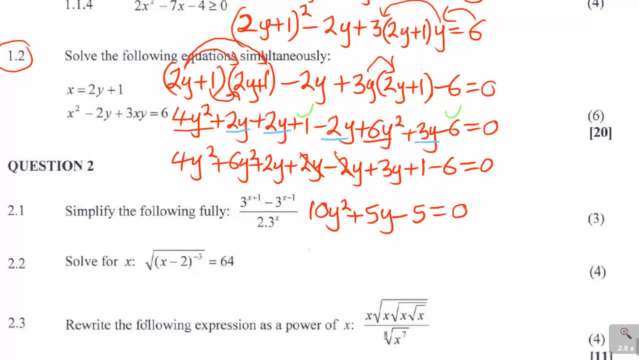 equation straight away, like that, because this is: you can divide by 5 if you want, but it's not a must. you can use the quadratic equation. you can see this is a x squared plus bx plus c is equal to 0. so my a is 10. 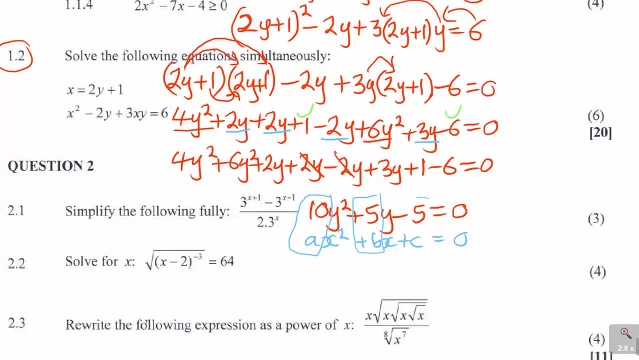 my b is 5 and my c is negative 5.. so what i will have is: y is equal to minus b, plus or minus square root of b, squared minus 4ac all over 2a i. i hope you are getting that. so, as i said, 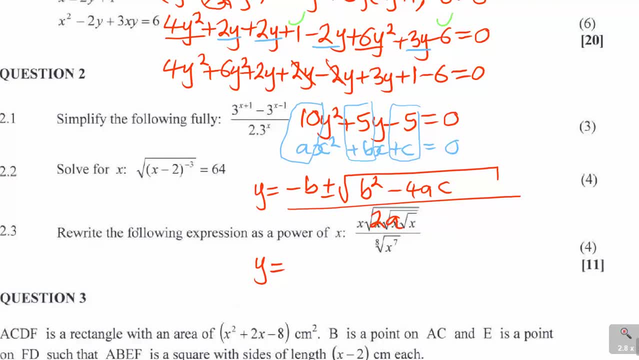 now you have to. i have those values to say what is your b? my b is 5 minus 5, plus or minus square root of 5, squared in brackets, minus 4. my a is 10. my c is negative 5 and then this thing is all over 2 and my a there is 10.. as i said, it's up to you. 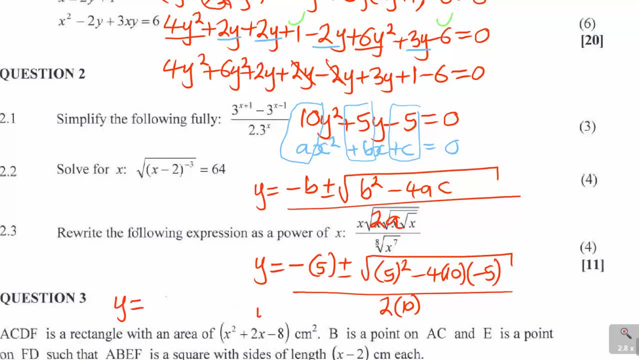 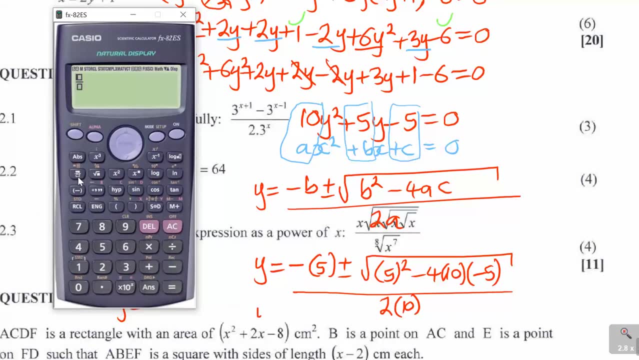 how you want to do it. so let's have two values of y. the first value of um of of y. if i use the calculator, i will have in this case minus 5. start with the positive square root of 5, squared in brackets: minus 4. my a is 10, my c is negative 5, and then this is all over 2. 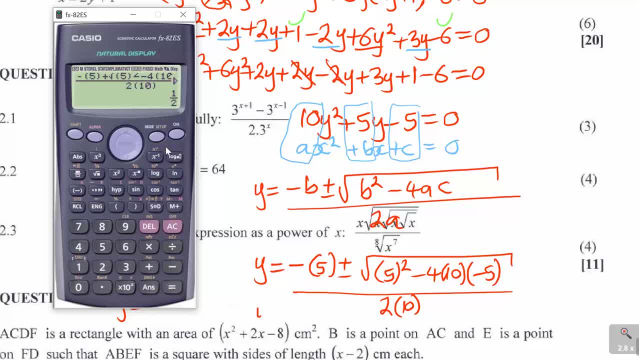 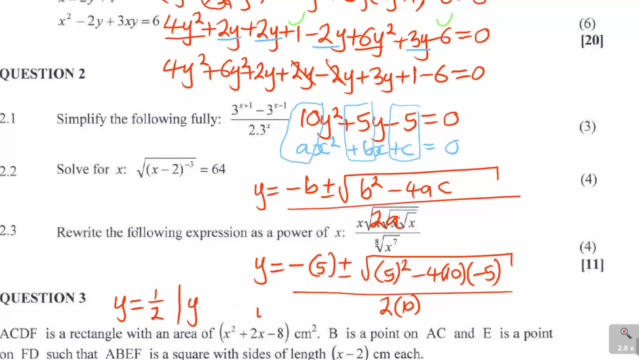 and my a is 10.. all right, so if i do that, my first value, y, is equal to a half or 0.5, and the other one, y, is called to negative 1.. so we have got y is equal to 1 over 2 or y is equal to negative. 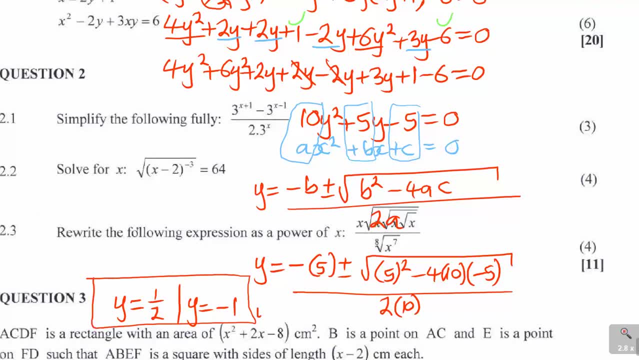 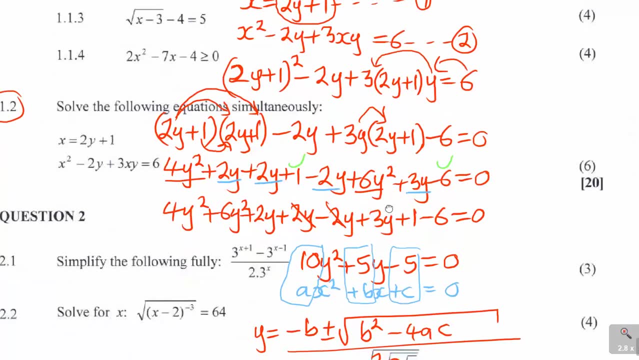 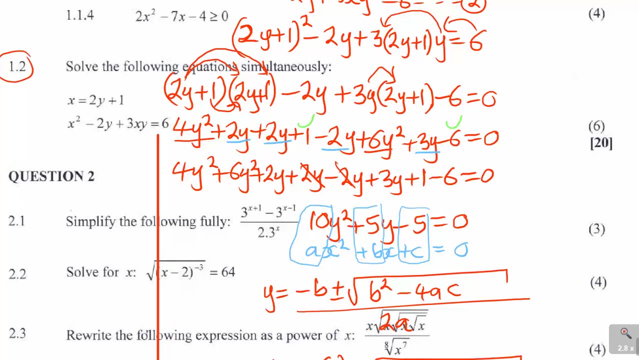 1.. so these are the two values of y that we got. but now i can go back to the equation, equation one. remember what we have in equation one. in equation one, um, if i can just work it, on the other side we had x is equal to 2y plus 1.. so where there is y, we have got two values of y. remember the other. 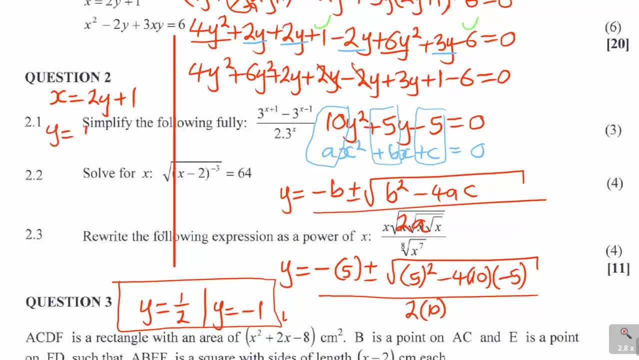 the first one is a half. so when you say, when y is equal to 1 over 2, so you have got x is equal to 2, 1 over 2 plus 1.. you can use a calculator that simplifies everything, or you can use your own knowledge. 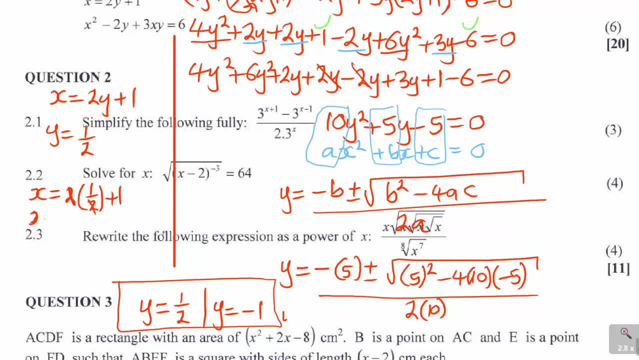 2 there, will cancel 2 there. so x is equal to 2 there. that's the first one. the second one is: yeah, you're quoting again the equation: x is 2y plus 1.. now, in this case, y is equal to negative 1, so x is equal to 2 minus 1 plus 1, so so 2 minus 1. 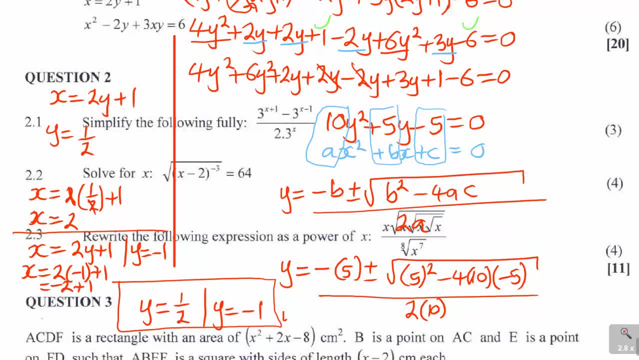 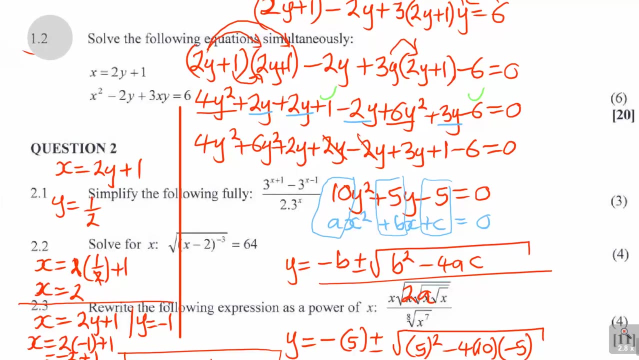 is equal to negative. 2 plus 1, which is equal to, so x is equal to negative 1.. so you have got two answers here. the first answer you must put it in, if i can erase this. so how do you present your final answers? you present them in kind of coordinates. 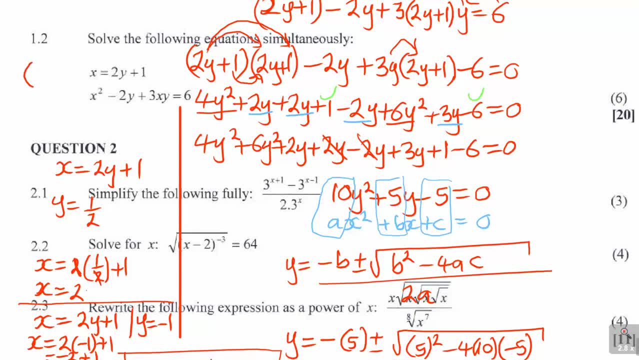 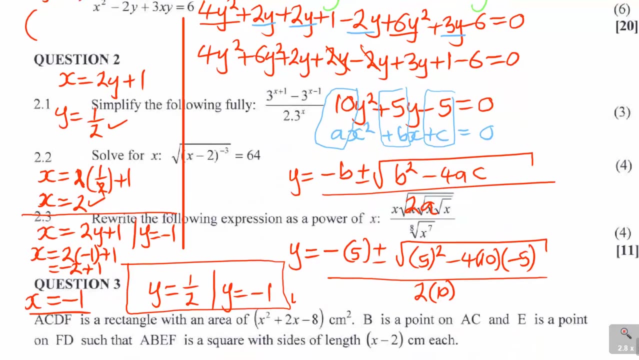 so the first one was when x was equal to 2, y was equal to half or 0.5, it's up to you how you want to present it. then the second one, when x was equal to negative 1. as you can see from here, y also was equal to. 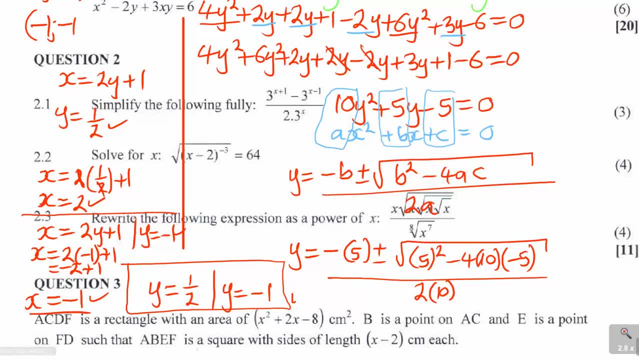 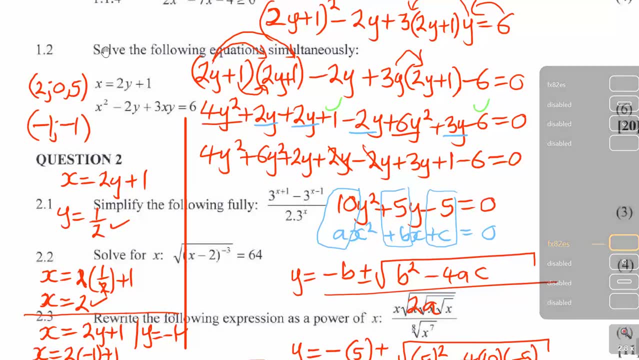 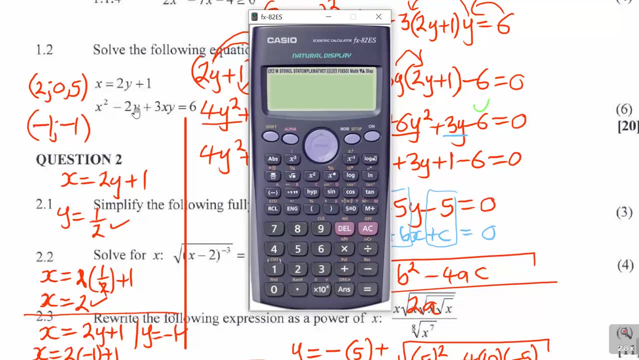 negative 1.. so that is how you can simplify such a question and get the answers, but now you definitely need to test them, and you must test them with the most um complicated one. you can see that the first one. don't test it with equation one, but go to equation two. and as you can see in equation two, where there 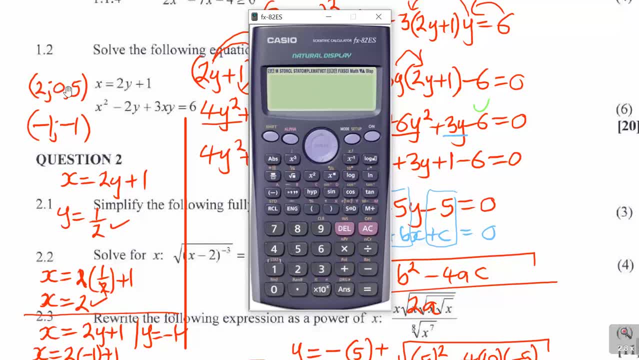 is x, you choose any pair. so where there is x, we can choose the first pair. it's 2, so it's bracket 2 squared right minus 2y, and then y is 0.5 and we have got plus 3, and where there is x we put a 2, where there is y is 0.5. if i put an equal sign, it must give me 6.. 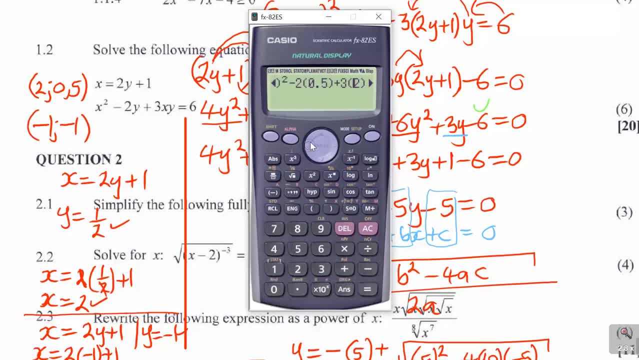 see i'm getting a 6. you can play backward on the same, but this time, whether is x- remember x- is now a negative 1, so you say minus 1 and then where there is y, which was 0.5, is also a negative 1. 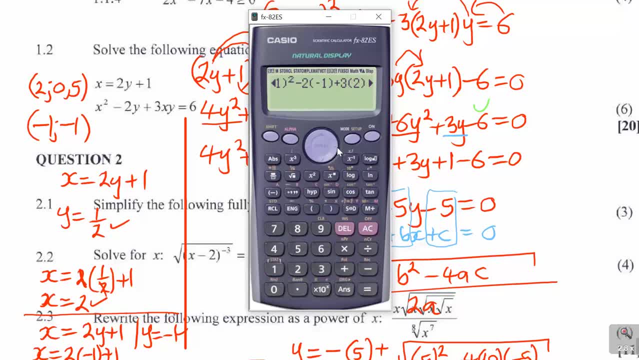 because x and y is negative 1, and then also the next one: where there is 2, i put a negative 1, and then where there is 0.5, i also put a negative 1.. so this must give me again a 6.. so you can see. 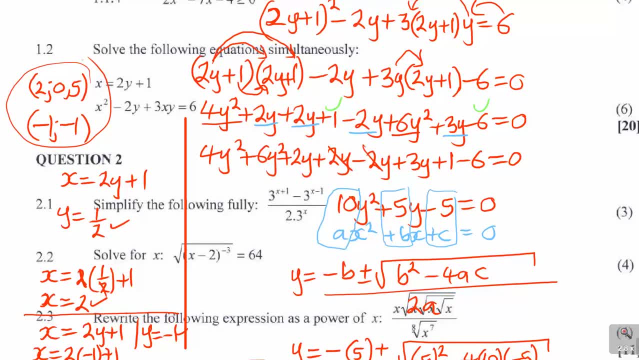 so it means my two values of x are correct. so that is how you approach a simultaneous equation. now, guys, i hope you benefited from this lesson as you are preparing for your final exams. i wish you all the best, but, more importantly, the most thing that i want you to emphasize here is: don't worry.